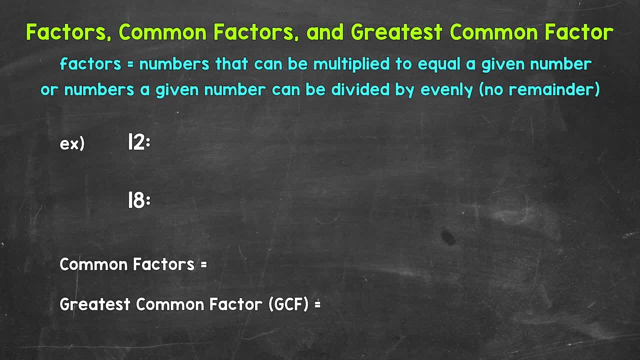 finding the greatest common factor of three numbers. After that we will take a look- at least common multiple. Now, when we think of factors of a number, we need to think what numbers can we multiply to equal that given number? Or what numbers can we divide that given number by evenly So divide with no remainder. 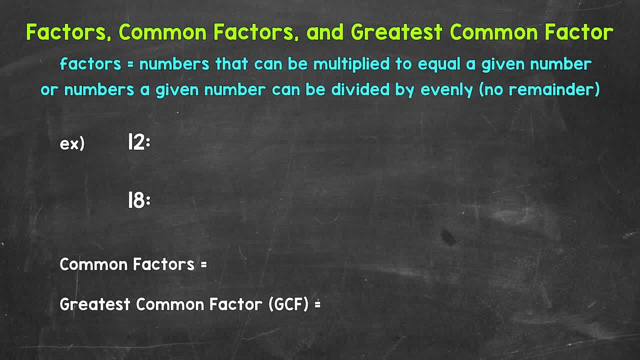 Now, it's not the most technical or mathematical way to word it, but you can think what numbers go into the given number. This will all make a lot more sense as we go through our example. Let's jump in. So let's jump into our example, where we have 12 and 18.. We're going to list the factors of 12 and. 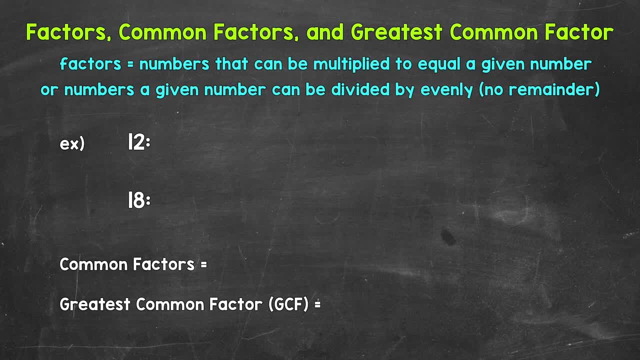 18, then find common factors and then, lastly, find the greatest common factor, which is also referred to as the GCF. Let's start with the factors of 12. And my suggestion would be to always start with 1 and the number itself. We can think of factors as the number itself, but we can also think of the 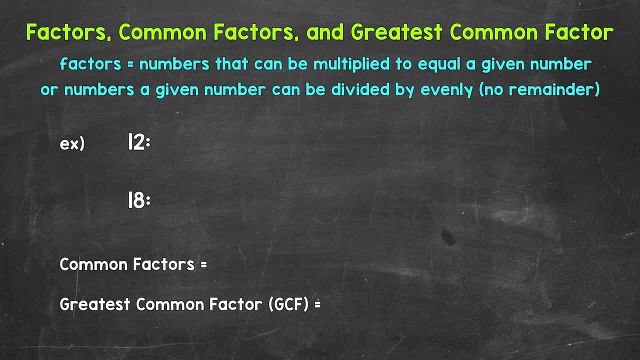 factors in terms of pairs. So 1 times 12 equals 12.. Or we can divide 12 by those factors, however you want to think about it. So I'm going to write 1 and 12 with a gap in between. That way we can. 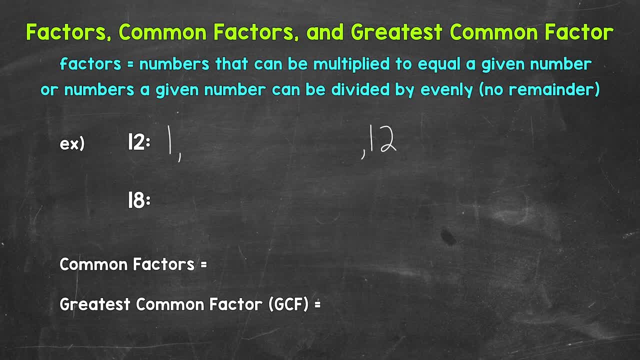 write the other factors in between 1 and 12, and we can write them in order. Now we need to list the other factors of 12.. So let's think of 12 as the number itself, and we can write the other factors. 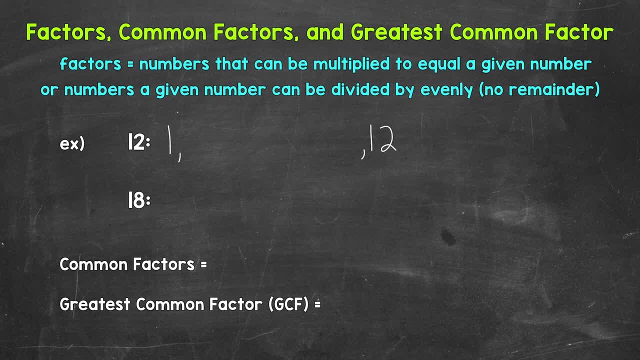 in terms of pairs. So let's think about what else goes into 12,, so to speak. Think of multiplication facts, division facts, and we can work our way up from 1.. So there are different strategies and ways to work through this. The next factors are 2 and 6.. 2 times 6 equals 12.. So 2 and 6 are factors of 12.. 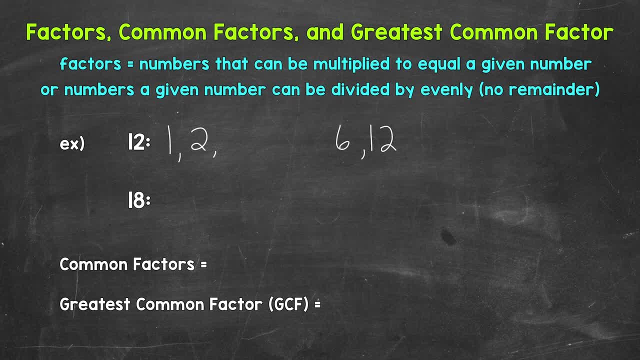 So 2 and 6. Then we have 3.. 3 and 4. 3 times 4 equals 12.. So 3 and 4 are factors of 12 as well, And again we can also think of these: 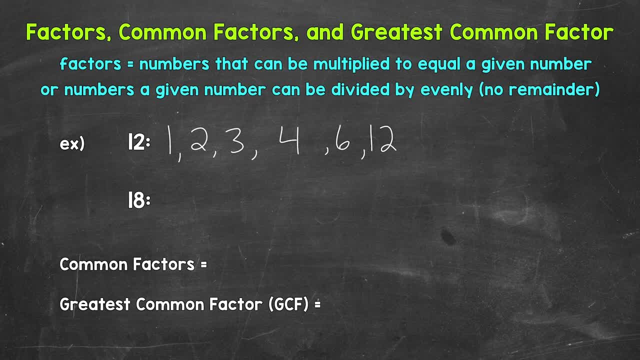 factors in terms of division, We can divide 12 evenly by these factors. Now, are there any more factors of 12?? No, We are done. That's our list of factors for 12.. Let's move on to the factors of 18.. 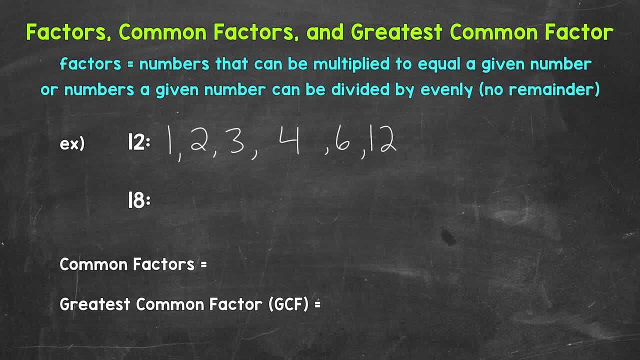 We will start. Let's start with 1 and 18.. So 1 and 18, with a gap in between. Next we have 2 and 9.. 2 times 9 equals 18.. So 2 and 9 are factors. Then we have 3 and 6.. 3 times 6 equals 18.. So 3 and 6 are factors of 18.. 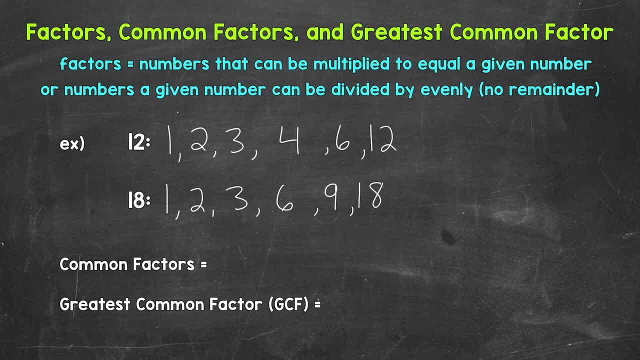 And that's it for the factors of 18.. Let's put the lists of there. You can always try more if you're unsure, if you have all of the factors. For example, we can think about 4,, 5,, 7,, 8, and so on. 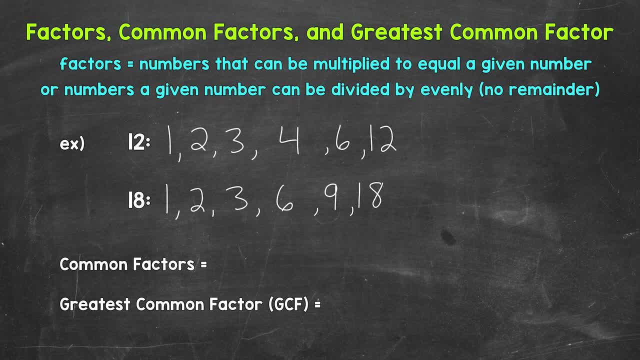 But we are done. That's our list of factors for 18.. One thing I do want to mention about factors and writing out these factor lists is that you will get better the more you do So writing the factors, the spacing of your lists. 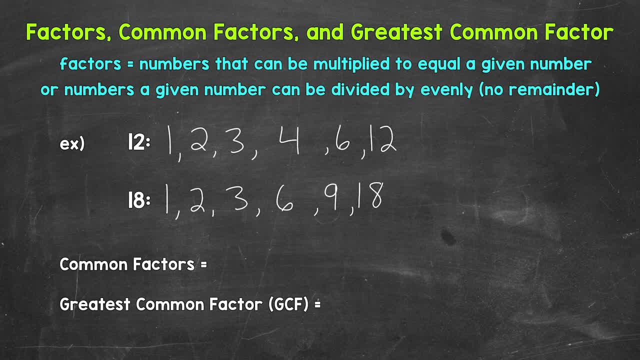 or whatever else the case be may be. So something to keep in mind. Now let's take a look at the common factors between 12 and 18.. That just means the factors they share, the factors they have in common. So 1 is a common. 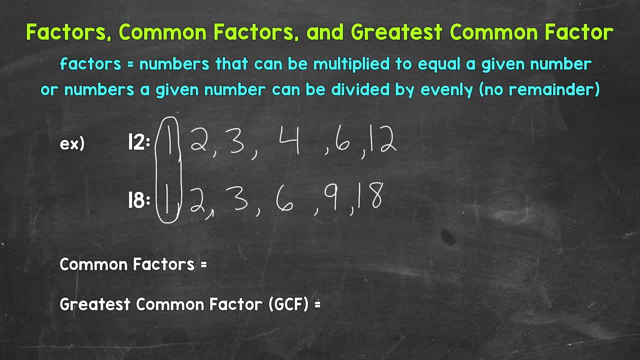 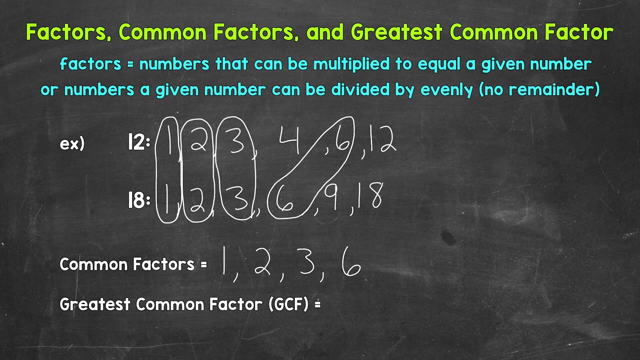 factor. 2 is a common factor, 3 is a common factor And then 6 is a common factor. So the common factors between 12 and 18 are 1,, 2,, 3, and 6.. Now we have the greatest common factor, or GCF. 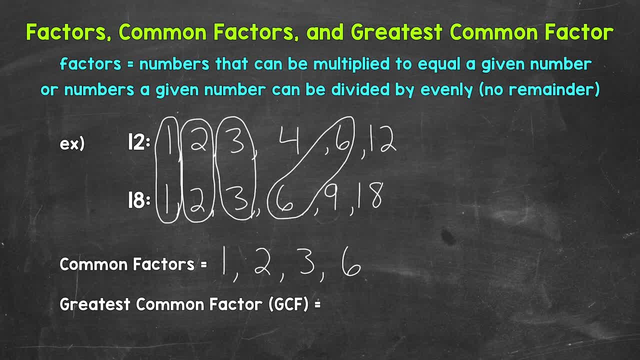 That's just the greatest factor in value that they share or have in common. The greatest common factor between 12 and 18 is 6.. So the greatest common factor equals 1. 6.. So there is an intro to factors, common factors and greatest common factor. Let's move. 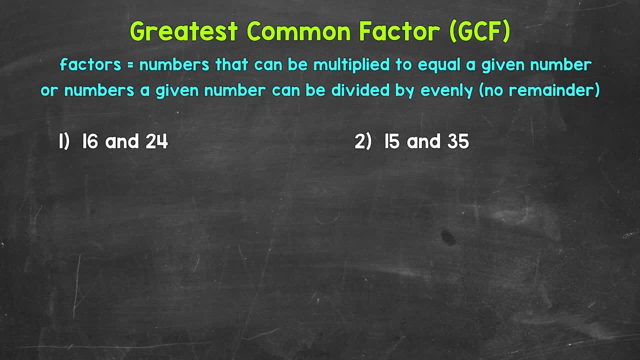 on to two more examples. Here are our next two examples and we will find the greatest common factor, just like we did in the intro, by listing the factors of the given numbers. So again, the greatest common factor is going to be the greatest or largest factor in value that both 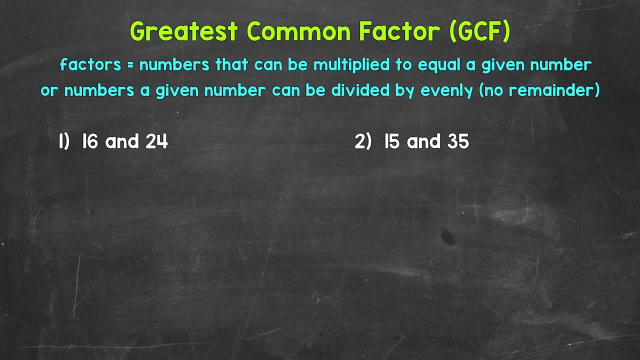 numbers share. Let's jump into our examples and see exactly what this looks like, Starting with number 1, where we have 16 and 24.. We first need to list the factors of each number. Let's start with the factors of 16.. Now I would suggest always starting with the factors of 1 and the number. 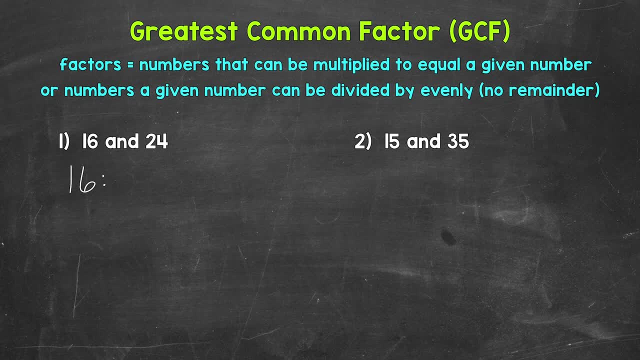 itself, Because we know 1 times that number will equal that number itself. We can think of factors in terms of pairs: 1 times 16 equals 16.. Or we can think of it in terms of division. We can divide 16 by those factors evenly, However you want to think about it. 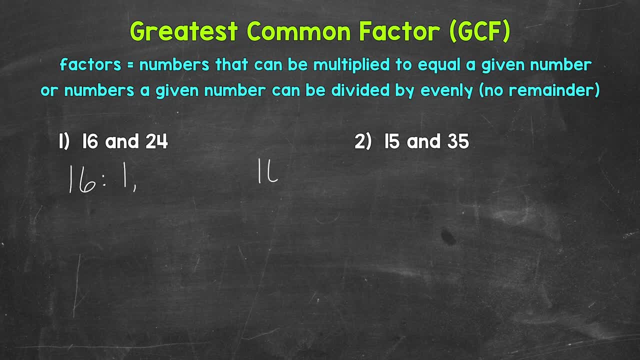 So I'm going to write 1 and 16, with a gap in between for the other factors. That way, we can divide 16 by those factors evenly. However you want to think about it, We can write the factors in order. Now we need to list the other factors of 16.. So let's think about: 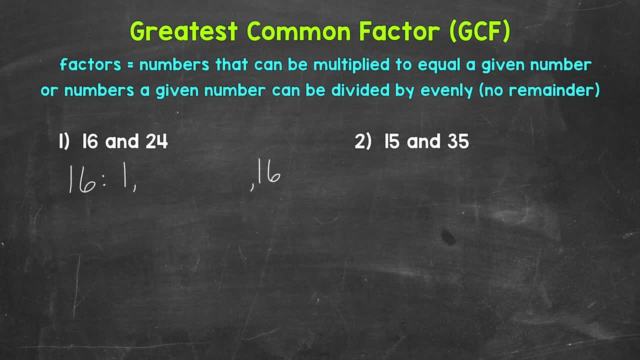 what else goes into 16,, so to speak. Think about multiplication facts, division facts, and we can work our way up from 1.. So there are different strategies and ways to work through this. The next factors of 16 are 2 and 8.. 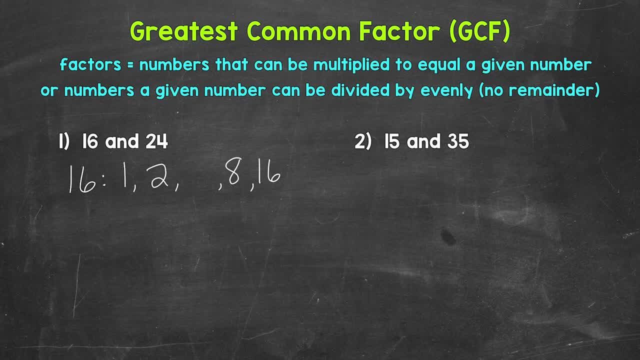 2 times 8.. 8 equals 16.. So 2 and 8 are factors of 16.. And then our last factor of 16 is 4.. 4 times 4 equals 16.. So 4 is a factor of 16.. Although 4 times 4 equals 16,, we only need to write 4 once. 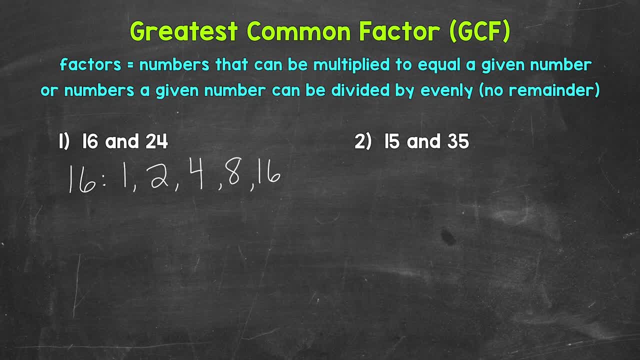 in our factors list. And that's it for the factors of 16.. You can always think about other possible factors If you're unsure, if you're done, for example, 3,, 5,, 6, and so on, But we have them all. 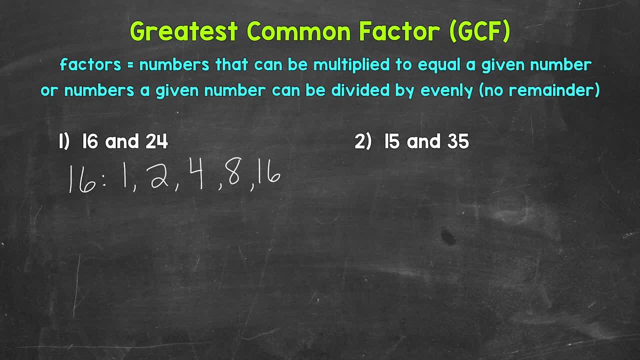 The factors of 16 are 1,, 2,, 4,, 8, and 16.. Let's move on to the factors of 24.. We will start with 1 and 24.. Next we have 2 and 12.. 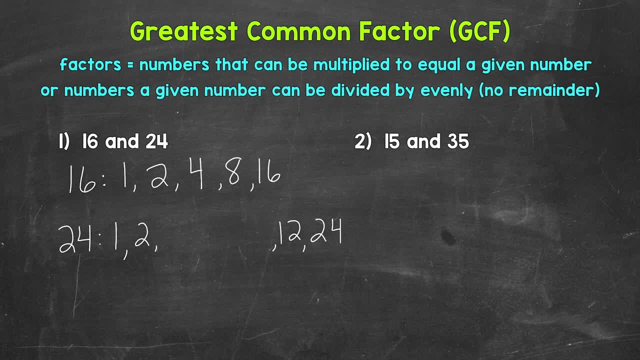 2 times 12 equals 24.. So 2 and 12 are factors of 24.. Then we have 3 and 8.. 3 times 8 equals 24.. So 3 and 8 are factors of 24.. And then, lastly, we have 4 and 6.. 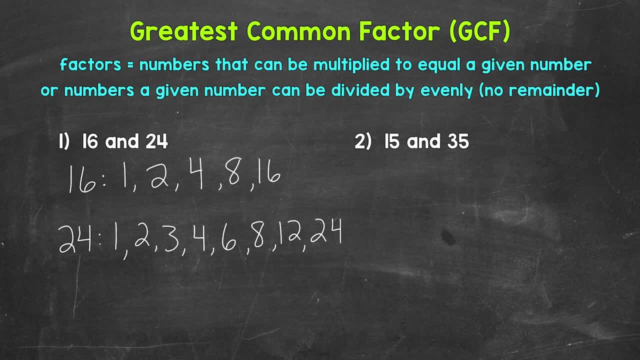 4 times 6 equals 24.. So 4 and 6 are factors of 24.. And that's it for the factors of 24.. 24.. 1,, 2,, 3,, 4,, 6,, 8,, 12, and 24.. Now that we have the factors listed for our numbers, we need to look. 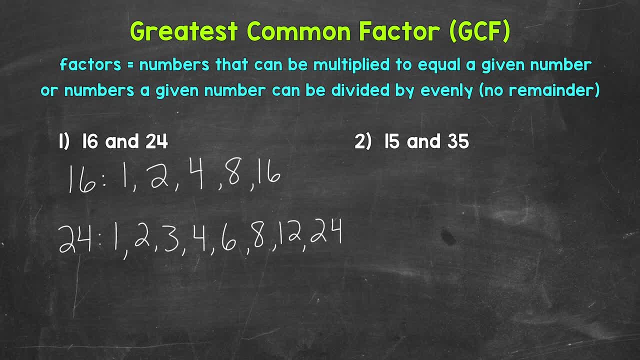 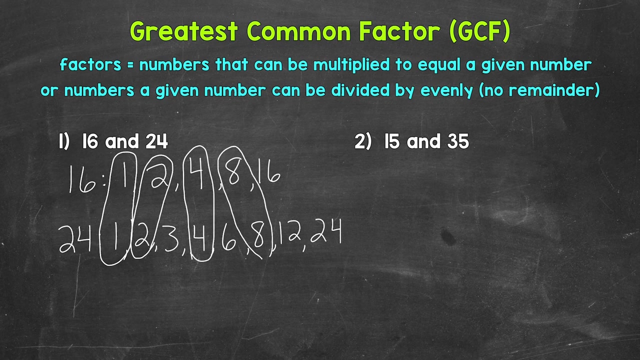 for common factors and specifically the greatest common factor. So let's look for factors that these numbers share, that they have in common. So 1 is a common factor, 2 is a common factor, 4 is a common factor And then 8 is a common factor. So the greatest common factor is 8,. 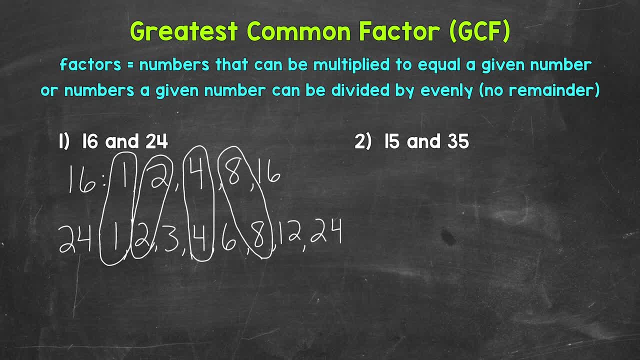 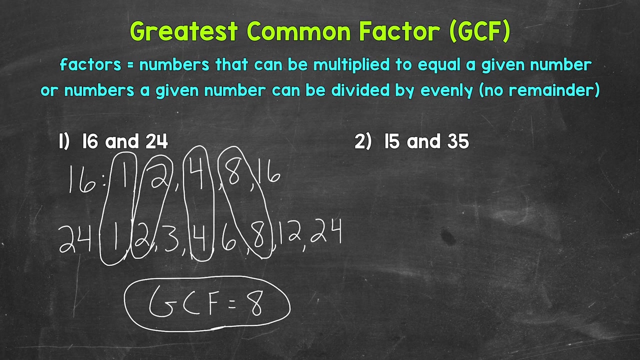 the greatest factor in value that they share, the greatest factor in value that they have in common. So the GCF, the greatest common factor is 8.. The greatest common factor of 16 and 24 is 8.. Let's move on to number 2, where we have 15 and 35. Let's start with the factors of 15.. 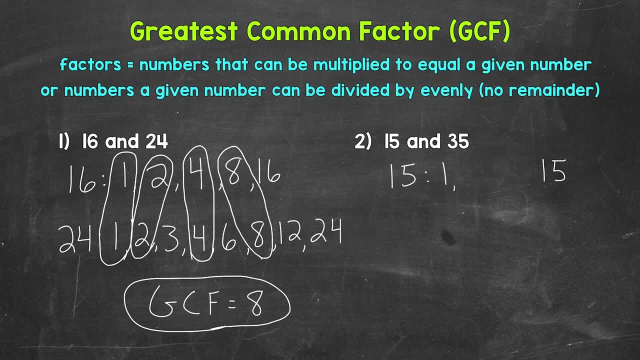 We have 1 and 15.. Next we have 3 and 5.. 3 times 5 equals 15.. So 3 and 5 are factors of 15.. And that's it for the factors of 15.. 1,, 3,, 5, and 15.. 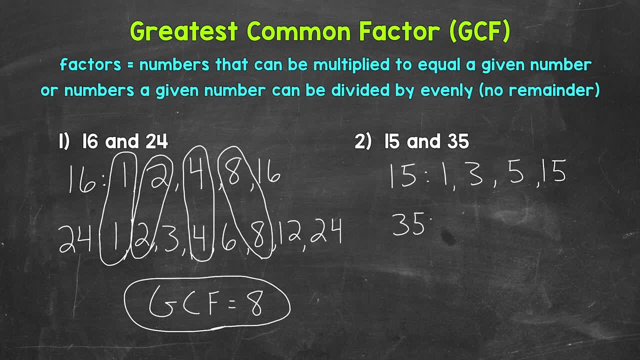 Now let's list the factors of 35. So we have 1 and 35, and then 5 and 7.. 5 times 7 equals 35. So 5 and 7 are factors of 35. And that's it. 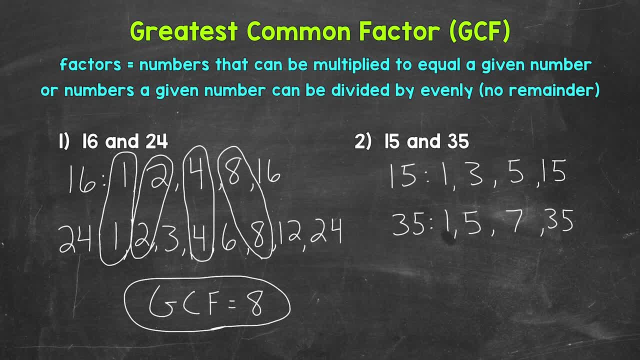 For the factors of 35.. 1,, 5,, 7, and 35.. Now that we have our factors list for our numbers, we need to look for common factors and specifically the greatest common factor. So 1 is a common factor And then 5 is a common factor. 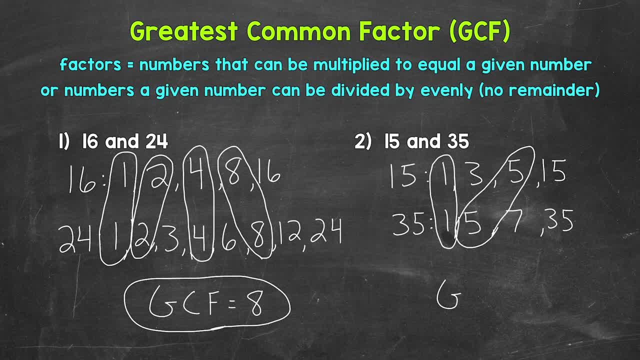 That means 5 is the greatest common factor. So the GCF, the greatest common factor is 5.. The greatest common factor of 15 and 35 is 5.. So there are two examples of finding the greatest common factor by listing the factors of the numbers. 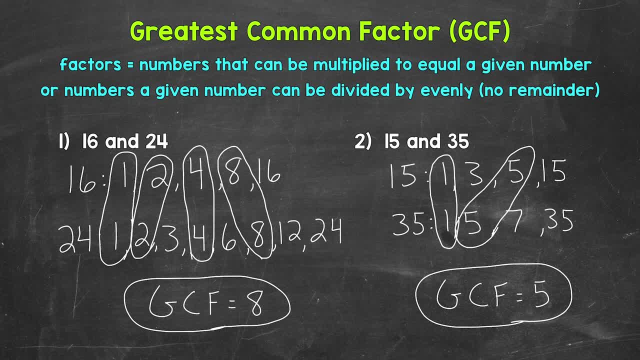 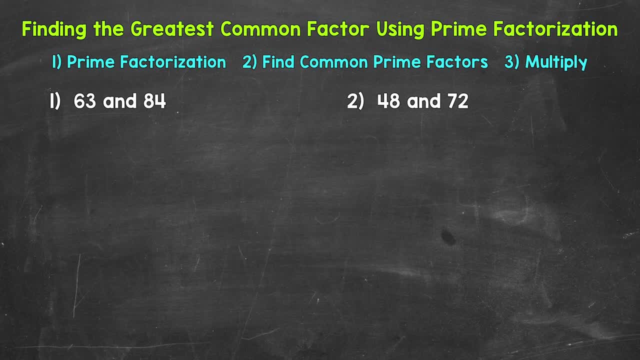 Let's move on to finding the greatest common factor using prime factorization. Here are our examples for finding the greatest common factor by using prime factorization. Now, I like using this strategy And find it helpful when working with numbers that are a little larger in value and not as simple to work with. 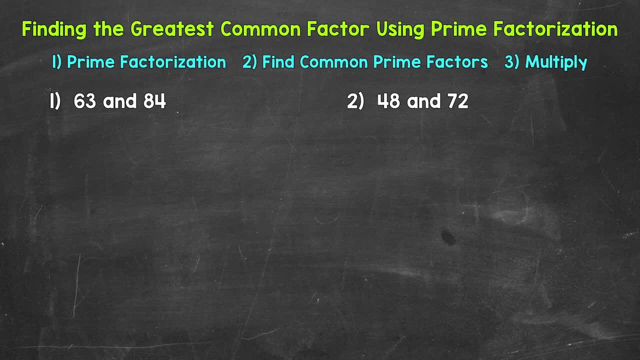 For example, the strategy of listing out all of the factors of the numbers in order to find the GCF can be kind of difficult and time-consuming when working with larger numbers in value. So this is a different approach, a different strategy to be familiar with when it comes to finding the greatest common factor. 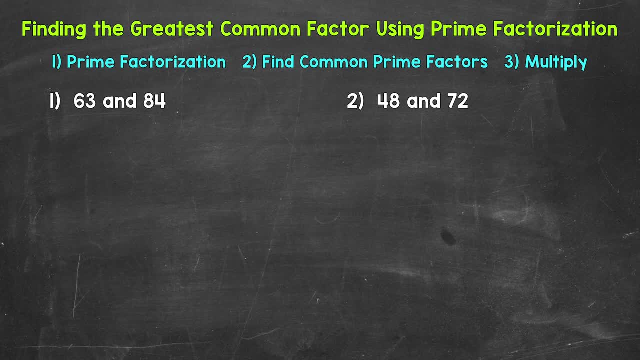 Let's jump in. Let's jump into our examples, starting with number 1, where we have 63 and 84.. Let's start with the prime factorization of 63. And we will start with the factors of 7 and 9.. 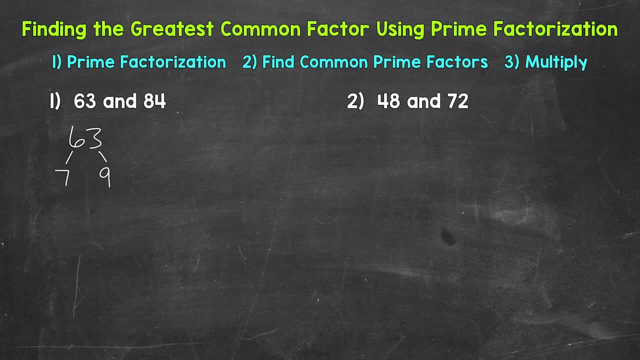 7 times 9 equals 63. So 7 and 9 are factors of 63.. Now 7 is prime, so we are done there. 9, we can break down 3 times 3, equals 9.. So 3 is a factor of 9.. 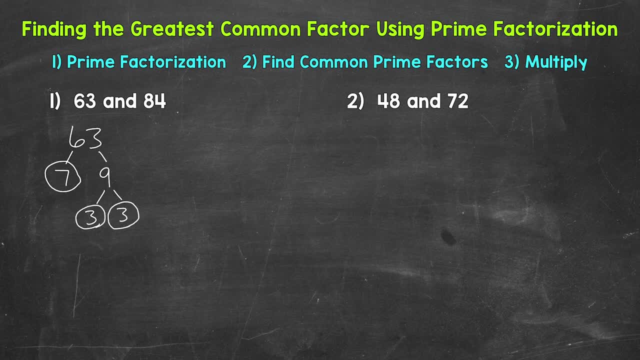 3 is prime. so we are done there and there, And that's the prime factorization of 63.. We can't break that down any further. Now we have the prime factorization of 84.. Let's start with the factors of 2 and 42.. 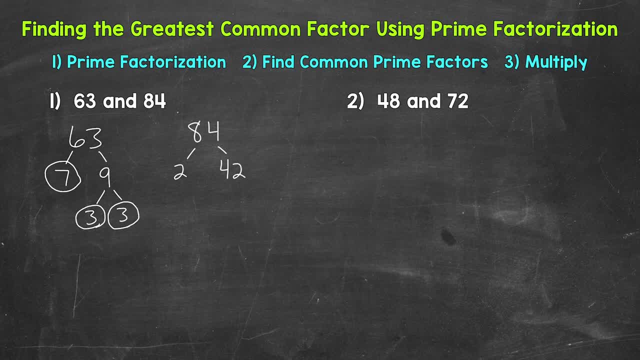 2 times 42 equals 84.. So 2 and 42 are factors of 84.. Now 2 is prime, so we are done there. 42, we can break down 2 times 21, equals 42.. So 2 and 21 are factors of 42.. 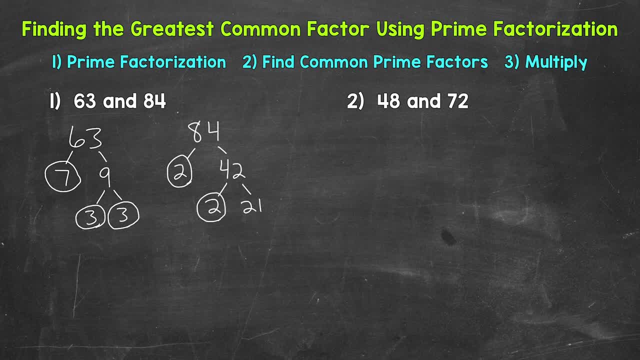 2 is prime. so we are done there. 21 we can break down: 3 times 7 equals 21.. 3 times 7 equals 21.. So 3 and 7 are factors of 21.. 3 is prime and 7 is prime as well. 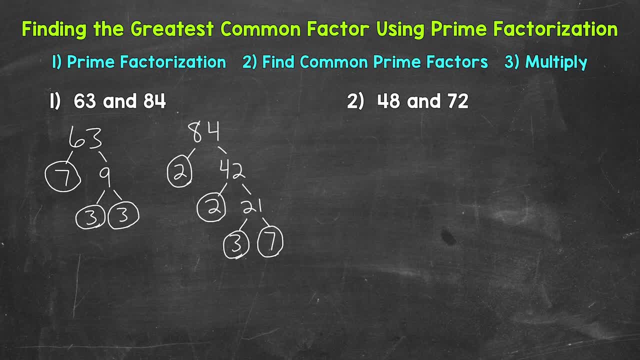 So we are done. That's the prime factorization of 84.. We can't break that down any further. Now that we have the prime factorization of both of those numbers, we need to find common prime factors, So prime factors that they share. 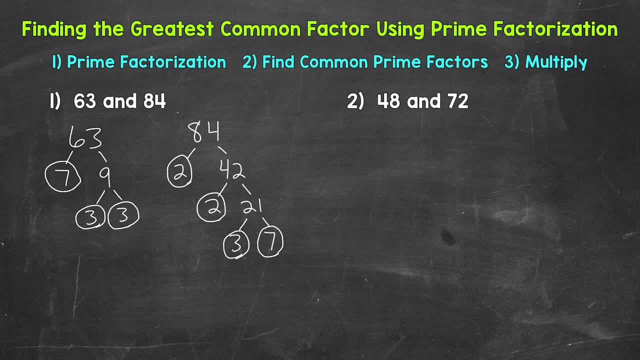 Now I'm going to list the prime factors of each to make it easier to find the ones that are common. So, as far as 63,, we have 3,, 3, and 7.. 3 times 3 times 7 equals 63.. 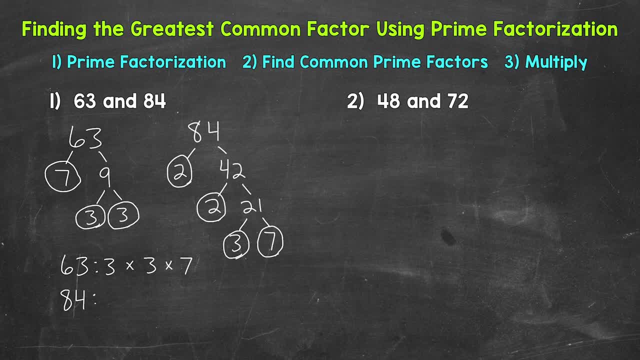 For 84,. we have 2,, 2,, 3, and 7.. 2 times 2 times 3 times 7 equals 84.. Now we need to find any common prime factors. 3 is a common prime factor. 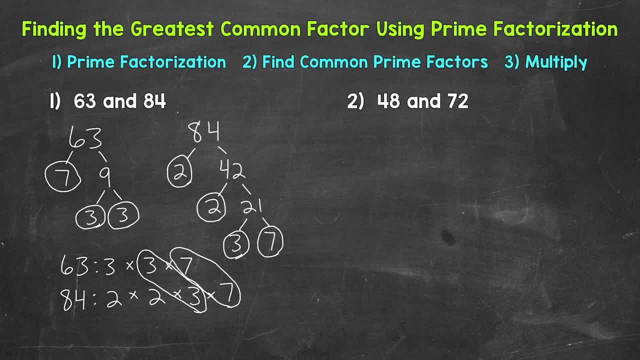 And 7 is a common prime factor, So they have a 3 and a 7 in common. Once we find those common prime factors, we multiply them, So 3 times 7, and that equals 21.. And that's our greatest common factor. 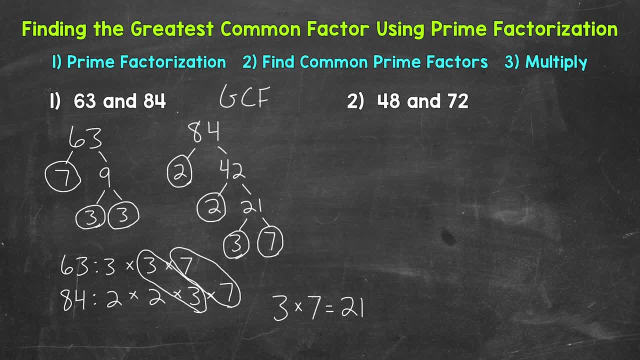 So the GCF- the greatest common factor of 63 and 84, is 21.. Let's move on to number 2, where we have 48 and 72. Let's start with the prime factorization of 48. And we will start with the factors of 2 and 24.. 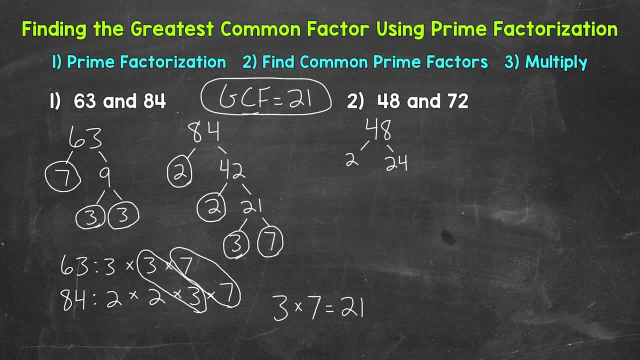 2 times 24 equals 48. So they are factors. Now, 2 is prime, so we are done there. We can break down 24.. 2 times 12 equals 24. So 2 and 12 are factors. 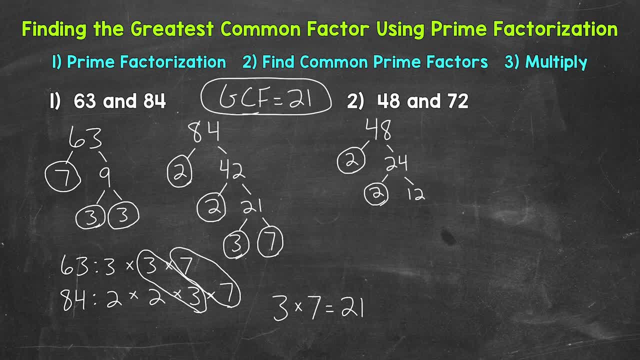 2 is prime, so we are done there. We can break 12 down further. 2 times 6 equals 12.. So 2 and 6 are factors. 2 is prime, so we are done there, But we can break 6 down further. 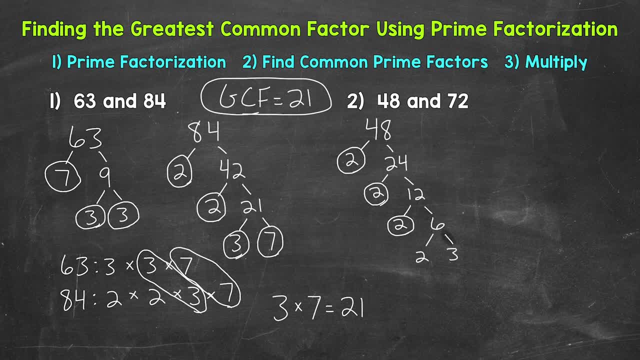 2 times 3 equals 6.. So 2 and 3 are factors. 2 is prime, so we are done there, And 3 is prime, so we are done there as well And we are done with the prime factorization of 48.. 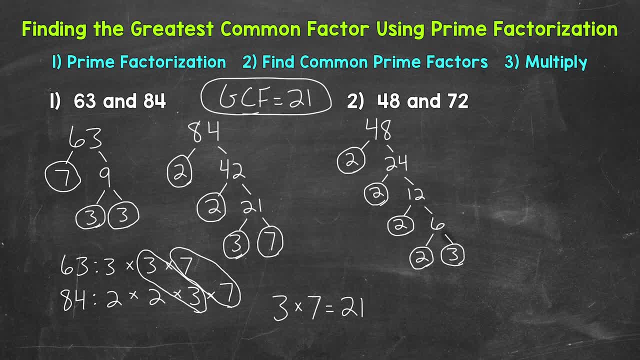 We can't break that down any further Now. we need the prime factorization of 72. Let's start with the factors of 2 and 36.. 2 times 36 equals 72. So they are factors, 2 is prime. so we are done here. 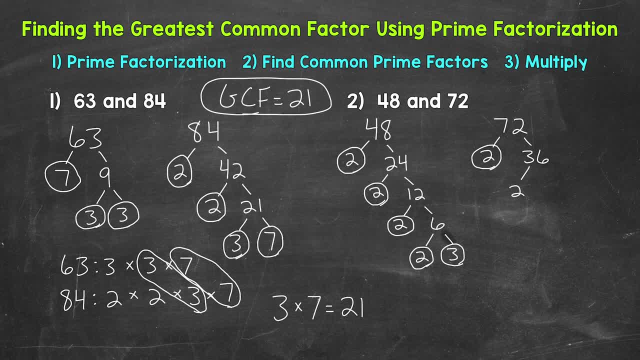 36, we can break down 2 times 18, equals 36.. So 2 and 18 are factors. 2 is prime. so we are done there. 18, we can break down 2 times 9, equals 18.. 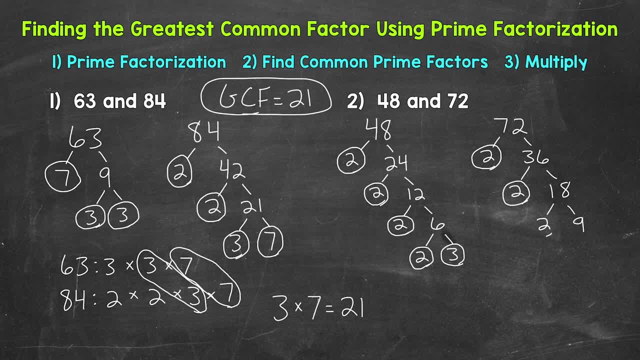 So 2 and 9 are factors. 2 is prime, so we are done there. But we can break 9 down further: 3 times 3 equals 9.. So 3 is a factor of 9.. 3 is prime, so we are done there. 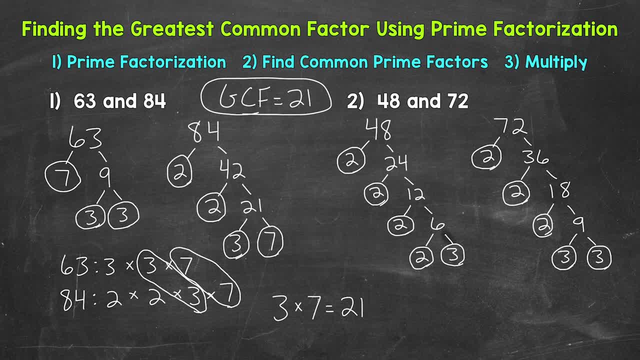 And there And we are done with the prime factorization of 72.. We can't break that down any further. Now that we have the prime factorization of both 48 and 72, we need to find common prime factors. So I'm going to write the prime factors of 48 and 72. 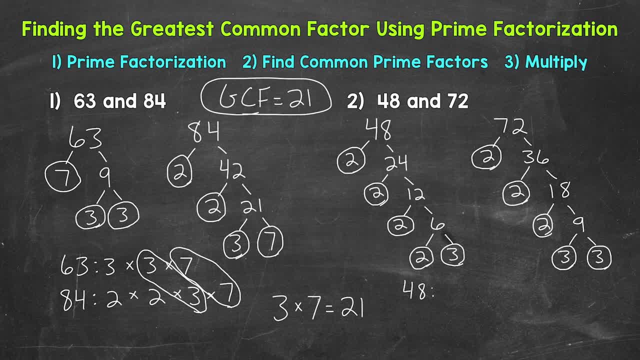 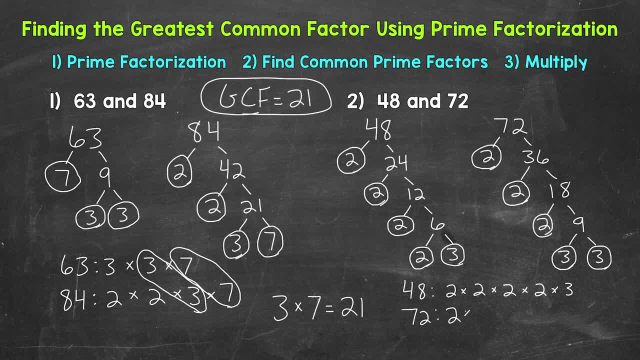 For 72, we have 2,, 2,, 2,, 2, 3, and 3.. 2 times 2 times 2 times 3 times 3 equals 72.. Now we need to find common prime factors. 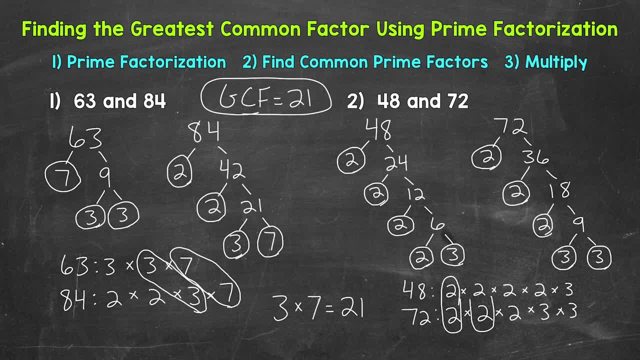 They have a 2 in common, another 2 in common and then a 3 in common. So now that we found the common prime factors, we need to multiply them to get the greatest common factor. So we have 2 times 2 times 2.. 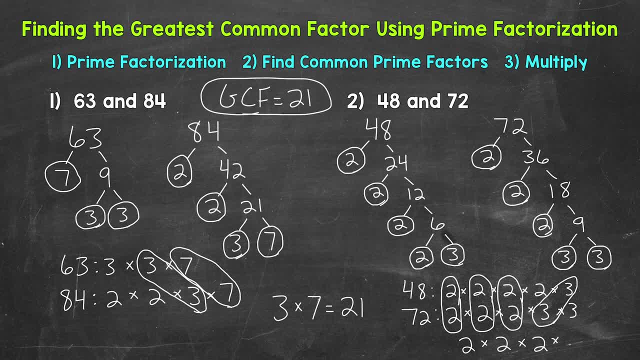 They have 3, 2s in common times 3.. 2 times 2 is 4 times 2 is 8 times 3.. 3 is 24.. So the GCF- the greatest common factor of 48 and 72, is 24.. 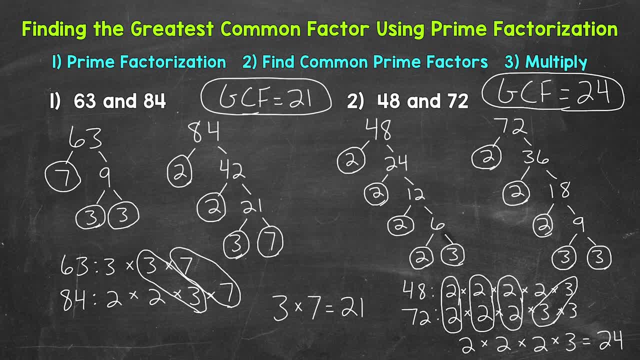 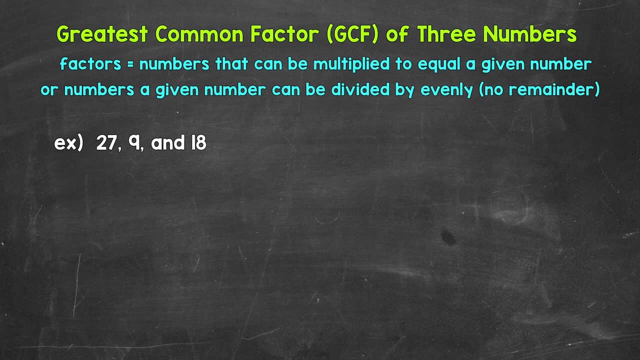 So there's how to find the greatest common factor using prime factorization. Let's move on to finding the greatest common factor of three numbers. Here is our example for finding the greatest common factor of three numbers, And in this example we will use the strategy of listing out the factors of the numbers. 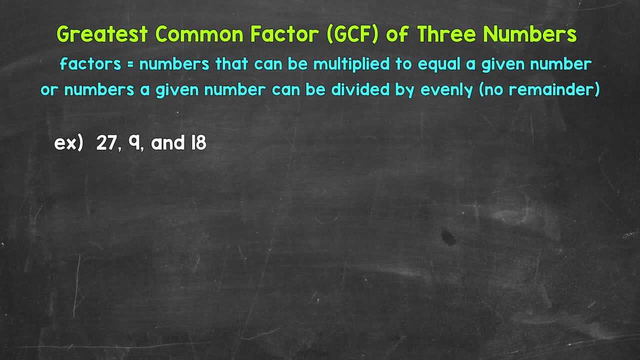 Let's jump into our example where we have 27,, 9, and 18.. We will start by listing the factors of each and then find the greatest common factor. Let's start with the factors of 27.. Now I would suggest always starting with the factors of 1 and the number itself. 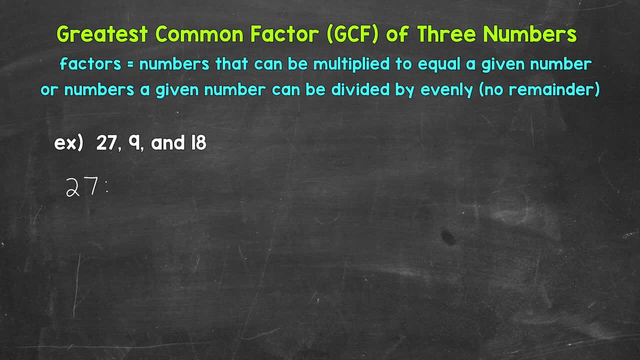 Because we know 1 times that number will equal that number itself. We can think of factors in terms of pairs: 1 times 27 equals 27.. Or we can divide 27 by those factors, evenly, However you want to think about it. 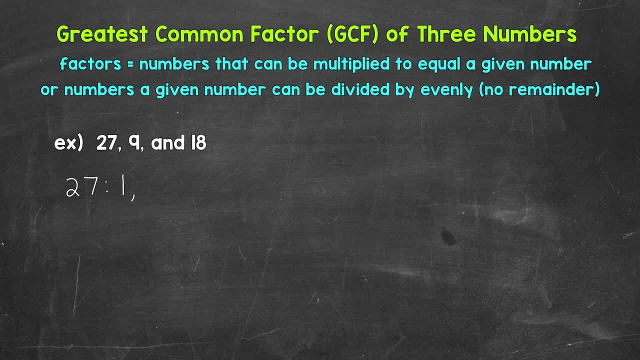 So I'm going to write 1 and 27, with a gap in between for the other factors. That way, we can write the factors in order. Now we need to list the other factors of 27.. So let's think about what else goes into 27,, so to speak. 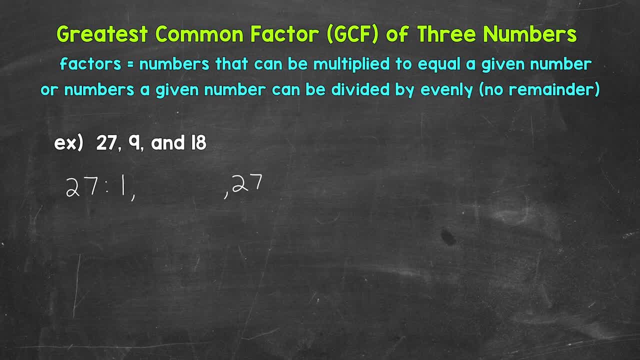 Think about multiplication facts, division facts, and we can work our way up from 1.. So there are different strategies And ways to work through this. The next factors of 27 are 3 and 9.. 3 times 9 equals 27.. 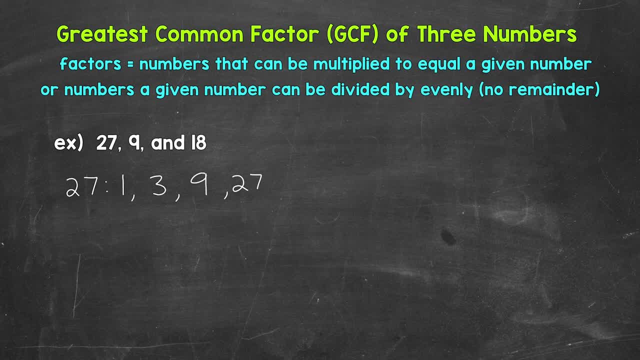 So 3 and 9 are factors of 27.. And that's actually it for the factors of 27.. You can always think about other possible factors if you're unsure, if you're done. For example, 2, 4.. 5, 6, and so on. 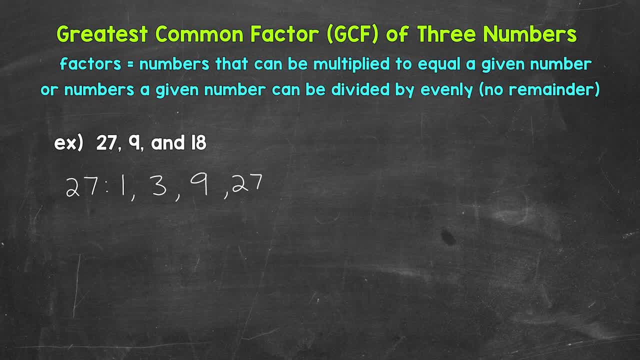 But we have them all: 1,, 3,, 9, and 27.. And, like I mentioned earlier, we can also think of these factors in terms of division. We can divide 27 evenly by all of these factors. Now, one thing I do want to mention about factors and writing out factors lists. 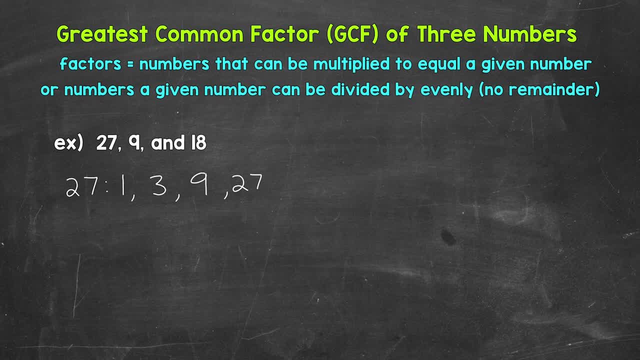 is that you will get a lot better the more you do Everything from writing and recognizing factors to the spacing of your lists. So something to keep in mind. Let's move on to the factors of 9.. And we can start with 1 and 9.. 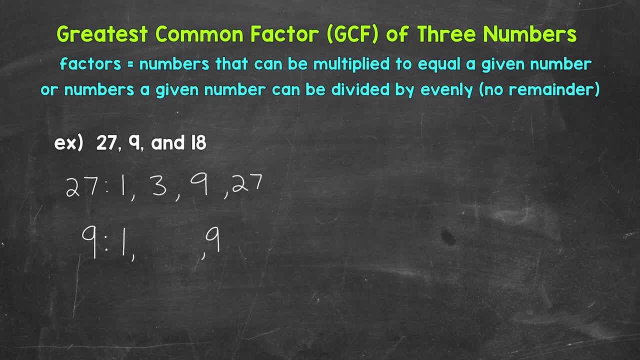 Now we need to think of other factors of 9.. Well, 3 times 3 equals 9.. So 3 is a factor of 9.. And although 3 times 3 equals 9, we just need to put 3 once there as far as the list of factors. 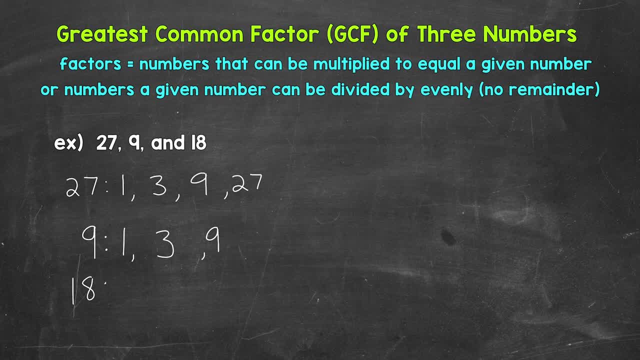 Lastly, let's list the factors of 18.. We can start with 1 and 18.. Next we have 2 and 9.. 2 times 9 equals 18.. So 2 and 9 are factors of 18.. 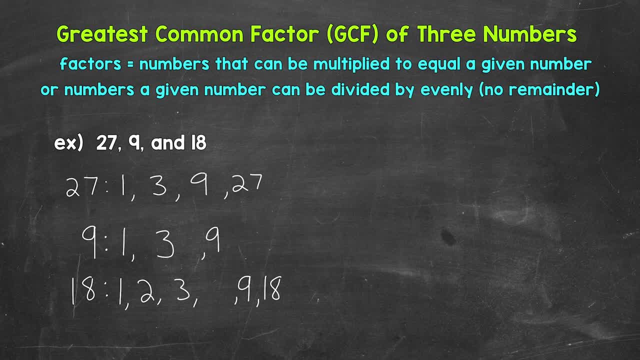 And then, lastly, we have 3,, 3 and 6.. 3 times 6 equals 18.. So 3 and 6 are factors of 18.. And that's it for the factors of 18.. 1,, 2,, 3,, 6,, 9 and 18.. 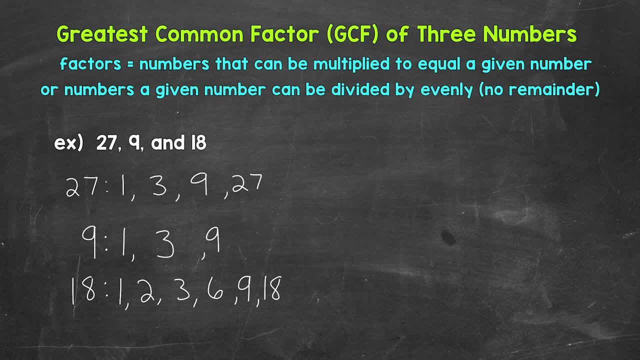 Now that we have all of the factors listed for our numbers, we need to look for common factors, So factors they share, And then, specifically, we need to look for the greatest common factor, So the greatest factor in value that they all share. 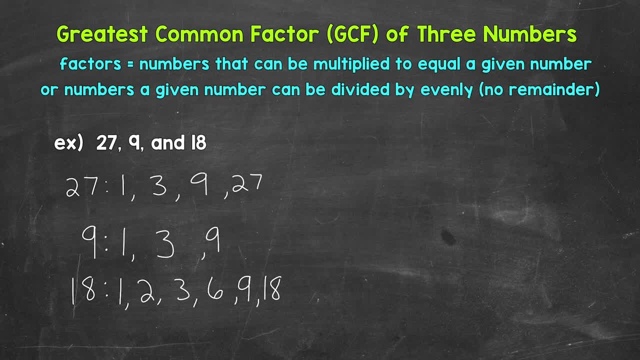 that they all have in common. So 1 is going to be a common factor, 3 is going to be a common factor And then 9 is going to be a common factor. So there are 3 common factors between these numbers. 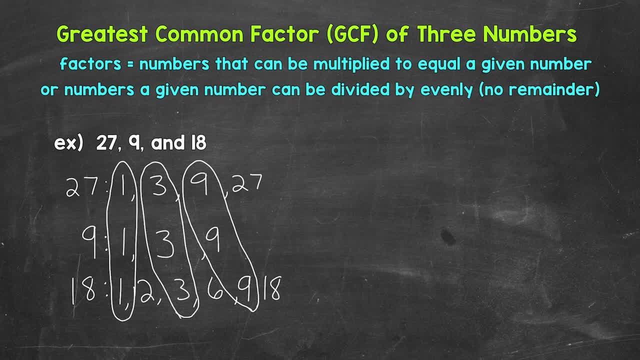 Now the greatest common factor is going to be 9.. So over to the right I'll write: the GCF, which stands for the greatest common factor, equals 9.. So the greatest common factor of these 3 numbers, 27,, 9 and 18,. 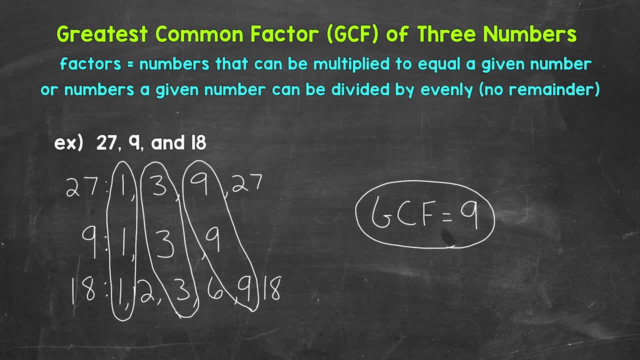 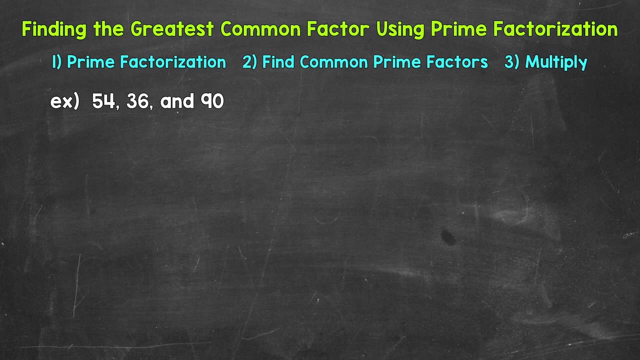 is 9.. So there's how to find the greatest common factor of 3 numbers: by listing the factors of the numbers. Let's move on to another example where we will use prime factorization. Here is our example for finding the greatest common factor of 3 numbers. 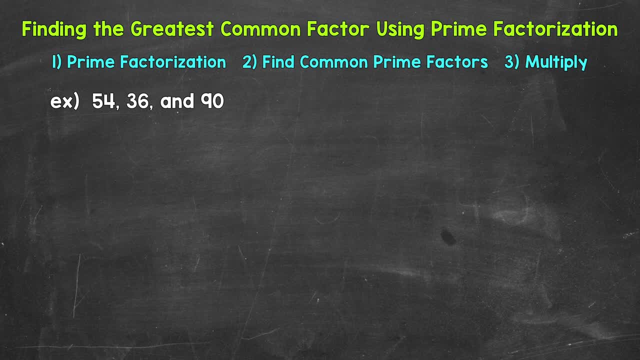 using prime factorization. Let's jump into our example where we have 54,, 36 and 90. So we need to find the greatest common factor of those 3 numbers. Let's start with the prime factorization of all 3 of our numbers. 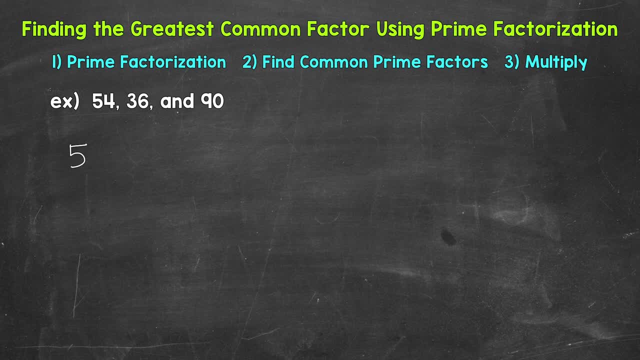 Starting with the prime factorization of 54.. 2 times 27 equals 54. So 2 and 27 are factors of 54. Now 2 is prime, so we are done there. 27, we can break down 3 times 9, equals 27.. 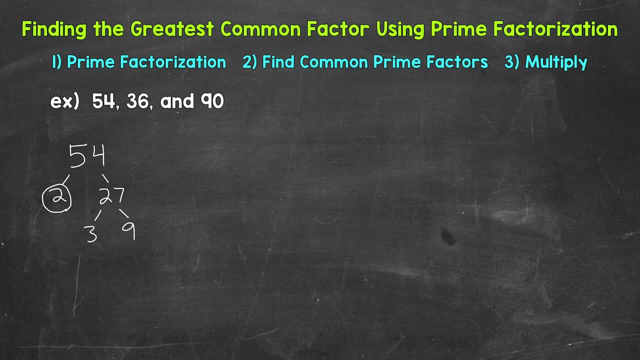 So 3 and 9 are factors of 27.. 3 is prime, so we are done there. 9, we can break down 3 times 3, equals 9.. So 3 is a factor of 9.. 3 is prime. 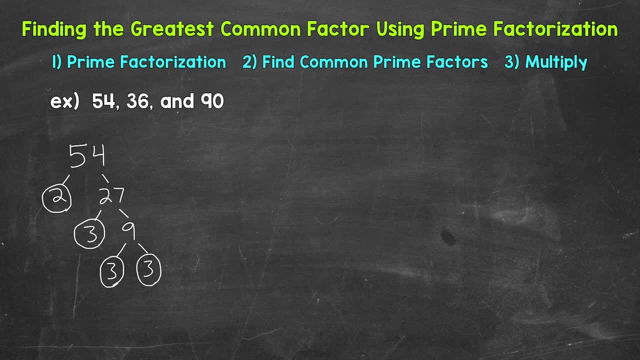 so we are done there and there, And that's the prime factorization of 54. We can't break that down any further. Let's move on to the prime factorization of 36.. 2 times 18 equals 36.. So 2 and 18 are factors. 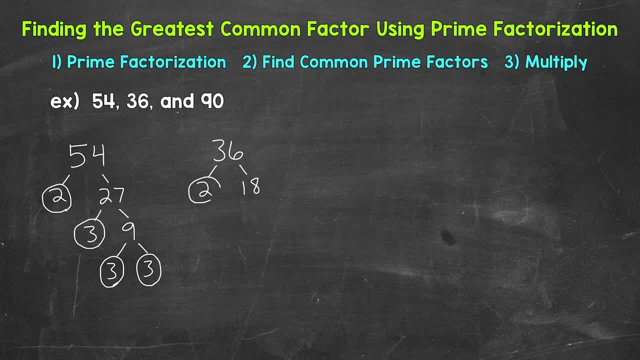 2 is prime, so we are done there. We can break 18 down further. 2 times 9 equals 18.. So 2 and 9 are factors. 2 is prime, so we are done there. We can break 9 down further. 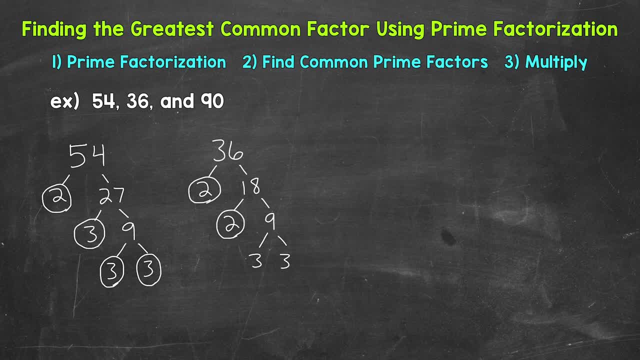 3 times 3 equals 9.. So 3 is a factor of 9.. 3 is prime, 3 is prime. so we are done there and there, and that's the prime factorization of 36. we can't break that down any further. and then, lastly, we have the 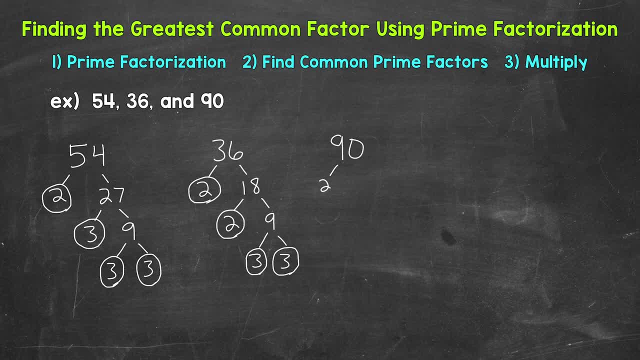 prime factorization of 90. 2 times 45 equals 90, so 2 and 45 are factors. 2 is prime, so we are done there. 45: we can break down further: 5 times 9 equals 45, so 5 and 9 are factors. 5 is prime, so we are done there. 9: we can break down 3. 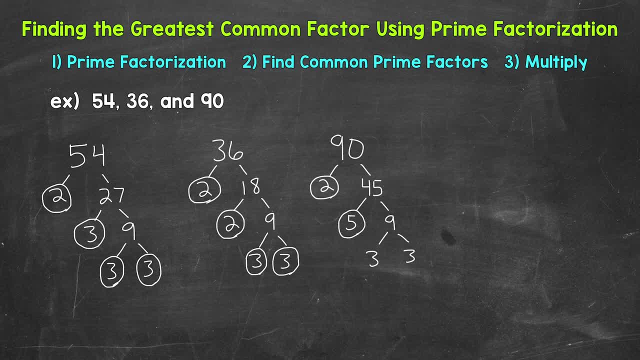 times 3 equals 9, so 3 is a factor, 3 is prime. so we are done there and there and that's the prime factorization of 90. we can't break that down any further. now that we have the prime factorization of all three of our numbers, we need to look for common prime factors. so prime 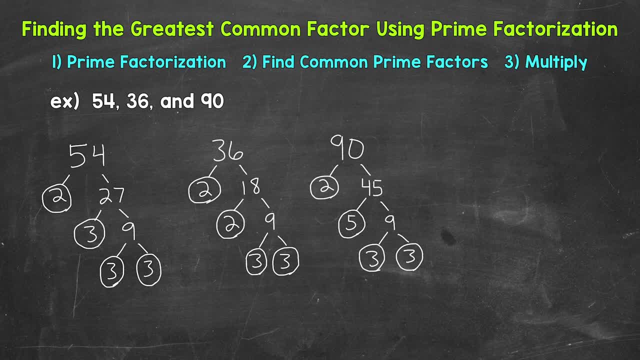 factors that all three of our numbers share, that they all have in common. now, in order to make it easier to find common prime factors, I'm going to list the prime factors off to the side here, starting with 54. so we have 2, 3 and. 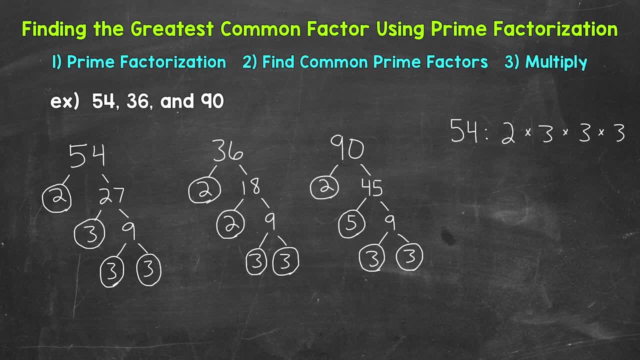 3 times 3 times 3 equals 54. now let's move on to 36. we have to 2,3,3, 2 times 2 times 3 times 3 equals 36, and then, lastly, we have 90. so 2, 3 and 3 times 3 equals 54negoo on XCB. lastly, we have 95, so 2x33, and again following the same O, is the prime factorization of 90, and 3 equals 54, equal to 35 new and 15 and in total of 45 dense xamsly, we have 32 die. 2,3,3 equals 56. and then, lastly, we have 90, 2, 2 and 3 two times 3: equalsторы equals 36, 26. and then, lastly, we have 90, 2 and 3 equals 24-3, 22 times 3 times 3. 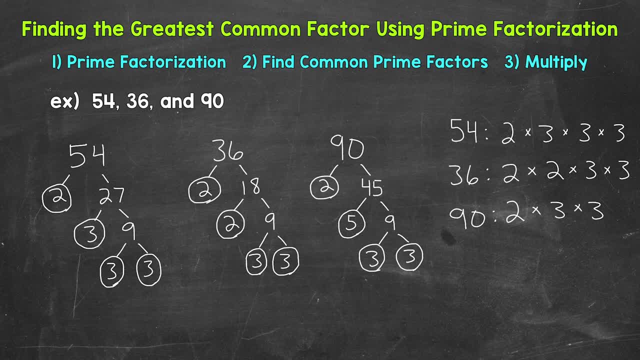 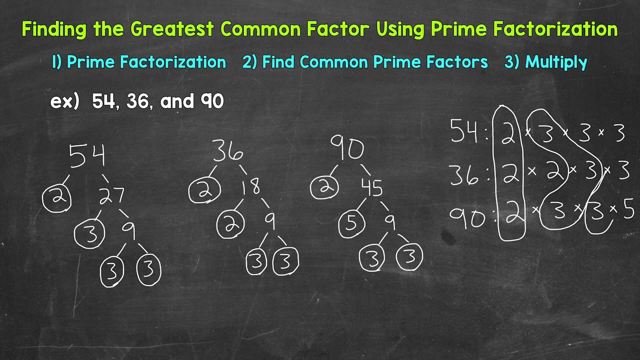 three, three and five. Two times three times three times five equals 90.. Now that we have the prime factors listed, we need to look for common prime factors, So factors that all three of these numbers share. So two is a common prime factor, three is a common prime factor, and then we have another three. 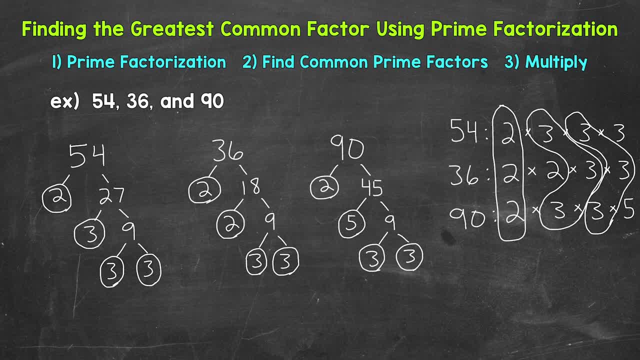 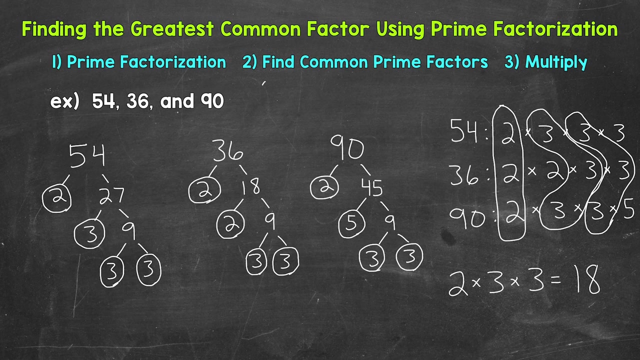 in common. The common prime factors are two, three and three. Now, once we have those common prime factors, we multiply them to get the greatest common factor. Two times three is six, times three is 18.. So the GCF, the greatest common factor of 54,. 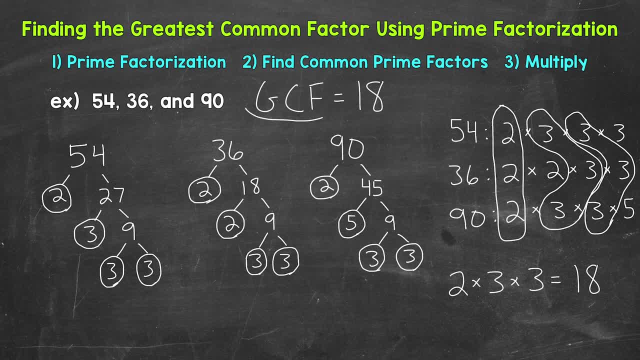 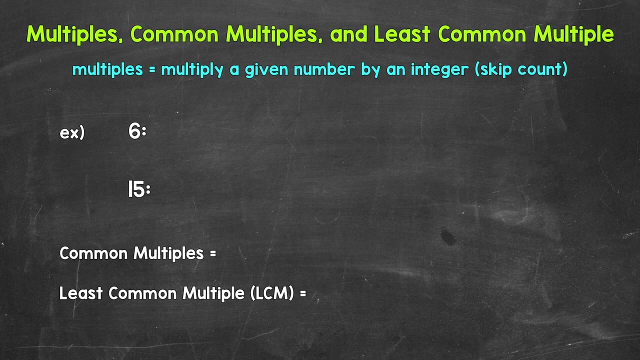 36, and 90 is 18.. So there's how to find the greatest common factor of three numbers using prime factorization, And that's a wrap for the greatest common factor portfolio. Let's move on to least common multiple. Let's start the least common multiple portion of this. 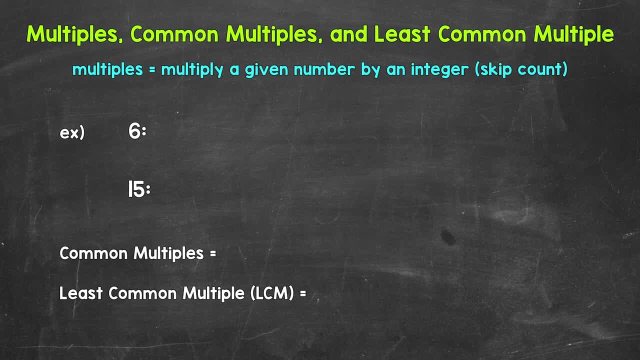 video with an intro. We will take a look at multiples, common multiples and least common multiple. So we will cover the basics in this section. Then we will move on to two more examples, followed by taking a look at a different strategy we can use to find the least common multiple. 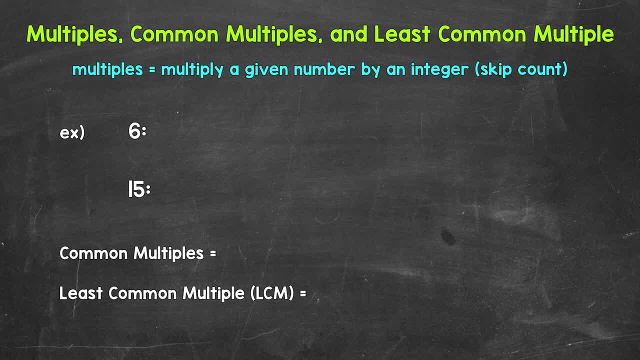 And then we will end with finding the least common multiple of three numbers. Now, a multiple is the result of multiplying a given number by an integer. So when we think of the multiples of a number, we need to think about the numbers we get when multiplying that given number by integers. A simpler way to think about: 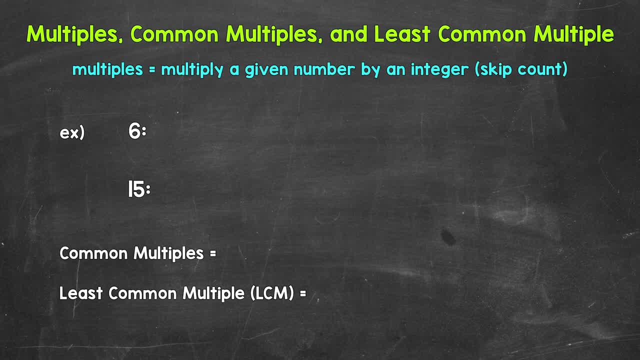 multiples is to think about skip counting. So all of the numbers, something is going to hit when you count up by that number. Those are all going to be multiples. This will make a lot more sense as we go through our example. Let's jump into our example where we have 6 and 15. We're going to 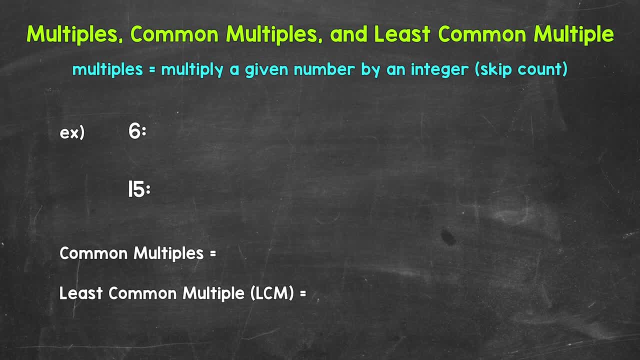 list some multiples of 6 and 15,, look at common multiples and then find the least common multiple, also referred to as the LCM. Let's start with the first 5 multiples of 6, which are 6 times 1,, which is 6.. 6 times 2 is 12.. 6 times 3 is 18.. 6 times 4 is 24.. 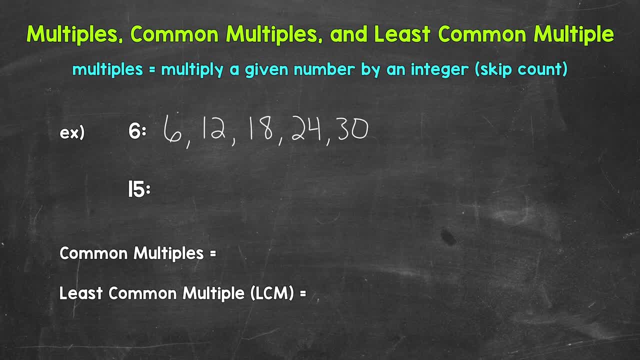 And 6 times 5 is 30. So those are the first 5 multiples of 6. And you can see that we just skip counted by 6.. 6,, 12,, 18, and 19.. So those are the first 5 multiples of 6. And you can see that we just skip counted by 6.. 6,, 12,, 18, and 19.. 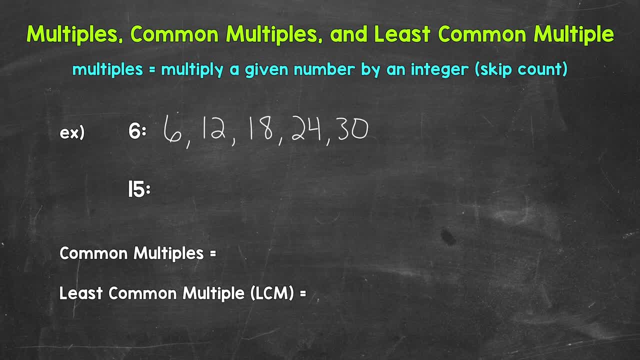 24,, 30, so on and so forth. Now I stopped at 30 because multiples go on forever. They are endless, They are infinite. My suggestion is to list 4 or 5 multiples when looking for common multiples or the least common multiple. 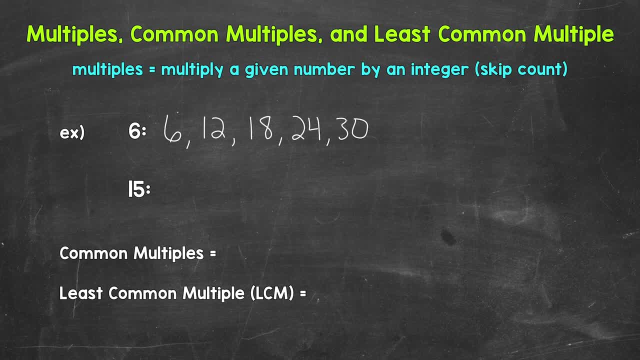 So list 4 or 5, look for any in common, and if you don't have any in common, you can always extend the multiples list. Now let's list the first five multiples of 15.. So 15 times 1 is 15,, 15 times 2 is 30,, 15 times 3 is 45,, 15 times 4 is 60, and then 15 times 5 is 75.. 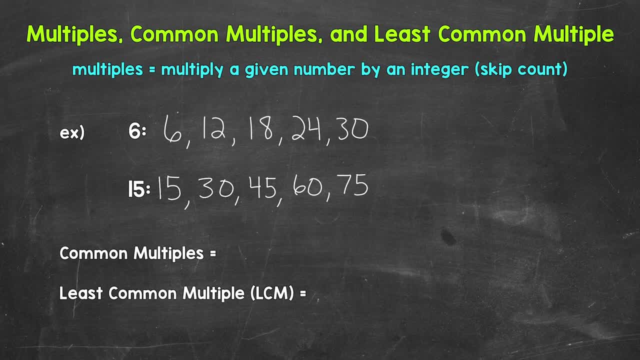 Now let's look for any common multiples, So any multiples they share, any multiples they have in common. Well, 30 is a common multiple. The next common multiple is 60. So let's extend the list of multiples for 6 there to show another common multiple. 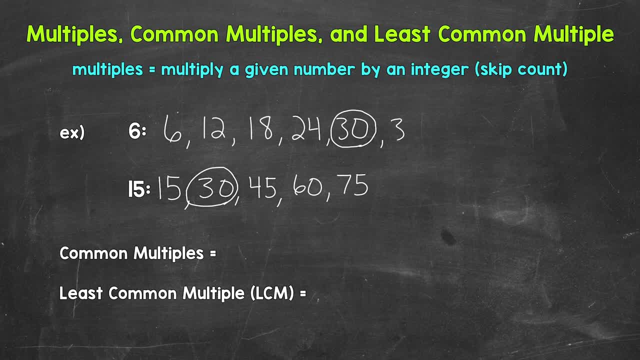 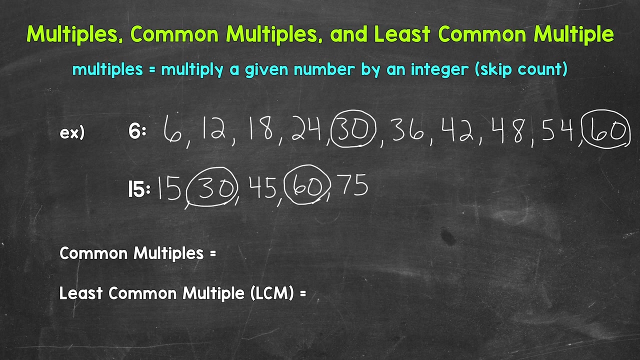 So after 30, we have 36,, then 42,, then 45.. 48,, then 54,, then 60. So another common multiple is 60. But again, remember, multiples lists go on forever. So we have an infinite amount of common multiples. 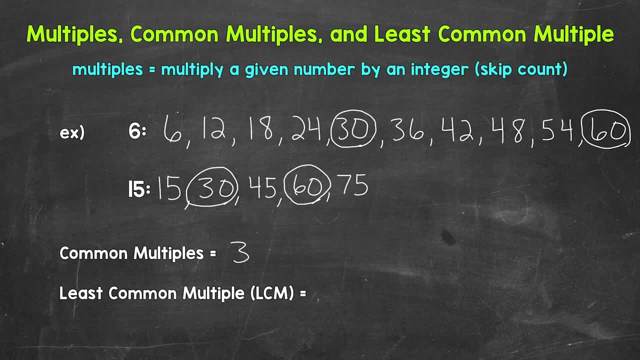 So down below for common multiples I'll put 30,, 60, and then make note that we have an infinite amount of common multiples. Now we have the least common multiple, which is just the smallest number in value that they have in common. 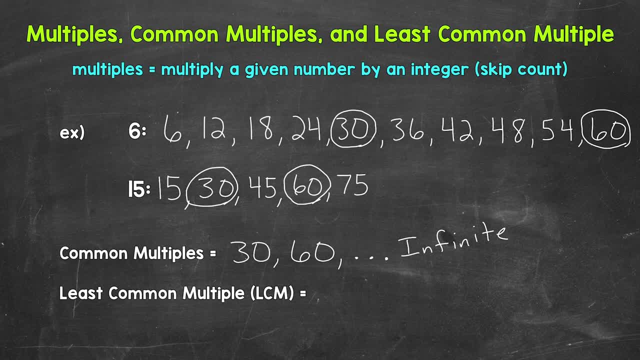 The smallest number in value that they share. This is going to be 30.. The least common multiple, or LCM, between 6 and 15 is 30.. So there's There's an intro to multiples, common multiples and least common multiple. 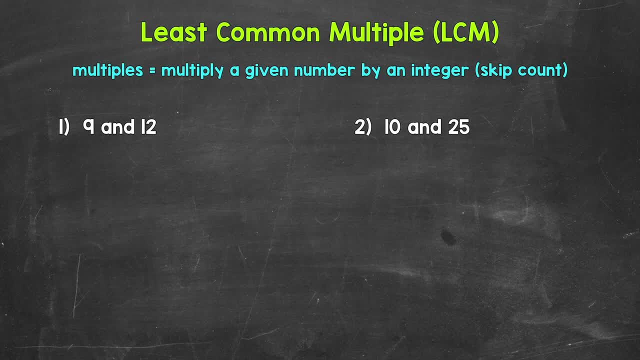 Let's move on to two more examples. Here are our next two examples, And we will find the least common multiple, just like we did in the intro by listing multiples of the given numbers. Now, as far as the least common multiple between numbers, this is going to be the smallest multiple in value that both 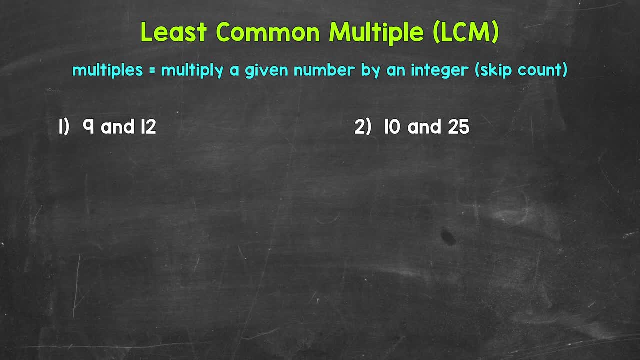 that both, that both numbers share. This will make a lot more sense as we go through our examples. Let's jump into our examples, starting with number 1, where we have 9 and 12.. We're going to start by listing some multiples of both 9 and 12.. 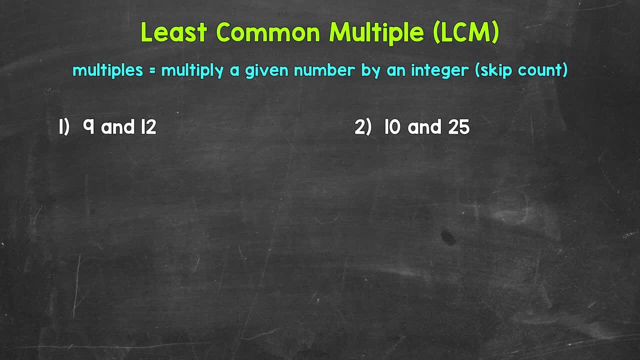 Then we will look for common multiples and specifically the least common multiple, also referred to as the LCM. Let's start with some multiples of 9.. Let's start with some multiples of 9.. Let's start with some multiples of 9,, which are 9 times 1,, which is 9.. 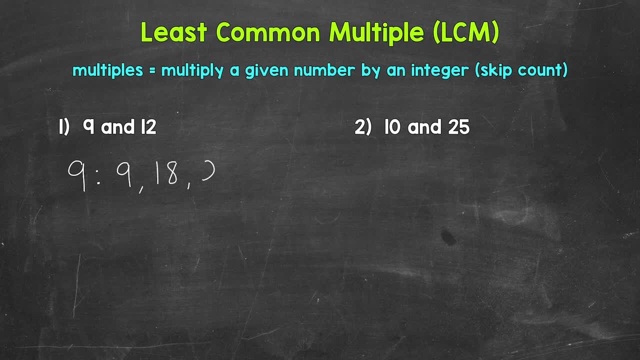 9 times 2 is 18.. 9 times 3 is 27.. 9 times 4 is 36.. And 9 times 5 is 45. So you can see that we just skip counted by 9 to list those multiples. 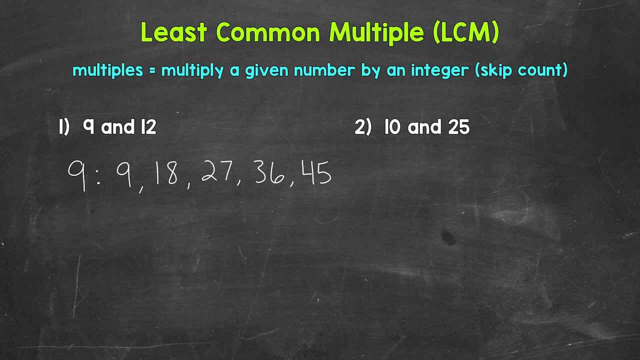 9,, 18,, 27,, 36,, 45,, so on and so forth. Now I stopped. Now I stopped at 45, because multiples go on forever, They are endless, They are infinite. My suggestion is to list 4 or 5 multiples when looking for the least common multiple. 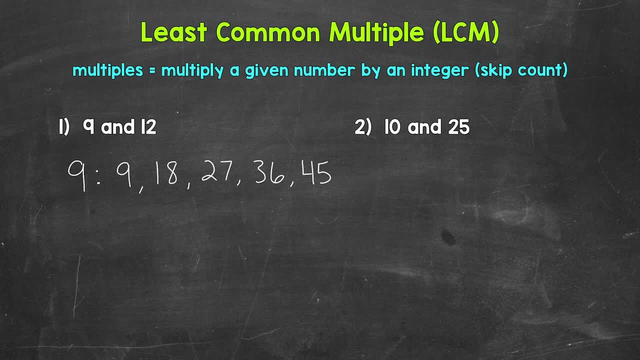 So list 4 or 5 multiples for each number. Look for any in common, And if you don't have any in common, you can always extend the multiples lists. Now let's list the first 5 multiples of 12.. 12 times 1.. 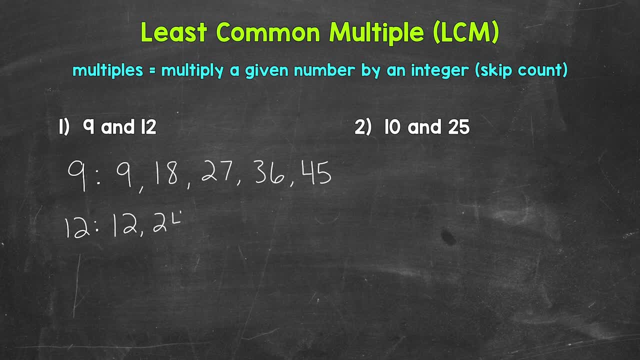 Is 12.. 12 times 2., Is 24.. 12 times 3., Is 36.. 12 times 4. Is 48. And 12 times 5. Is 60. So again you can see that we skip counted there. 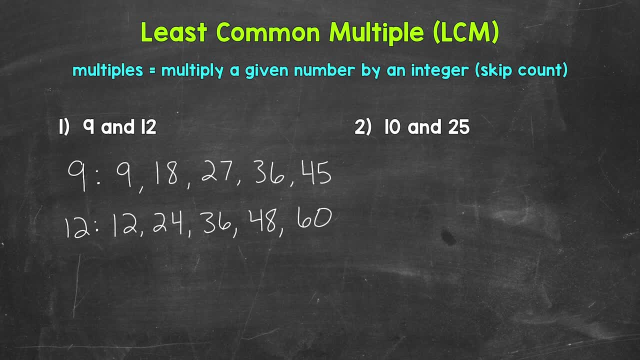 We skip counted by 12.. So 12,, 24,, 36,, 48,, 60, so on and so forth. Now that we have some multiples listed for both 9 and And 12, we need to look for any common multiples. 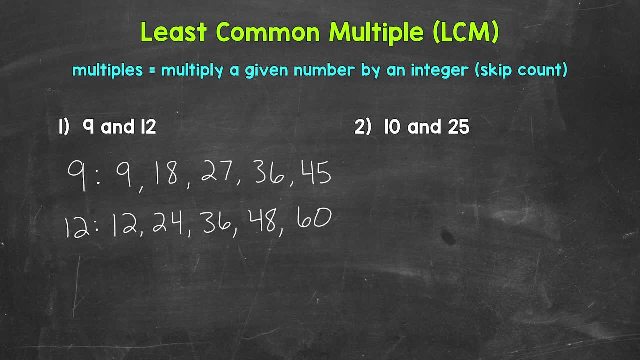 So any multiples that they share. And then, specifically, we need to look for the least common multiple. Well, 36 is a common multiple And it's going to be the least common multiple, So the smallest multiple in value that they share. 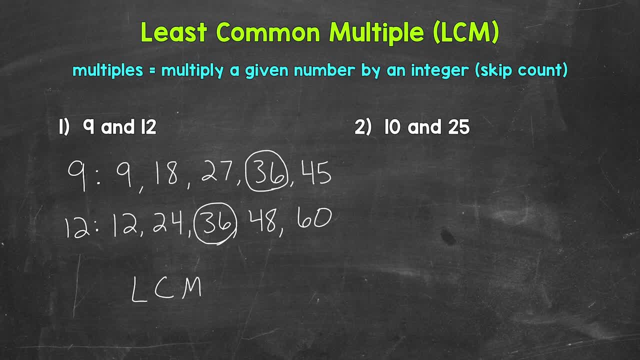 So let's write that the LCM, which stands for least common multiple, is 36.. So the least common multiple of 9 and 12 is 36.. Now, one thing I do want to mention about common multiples is that they are infinite. 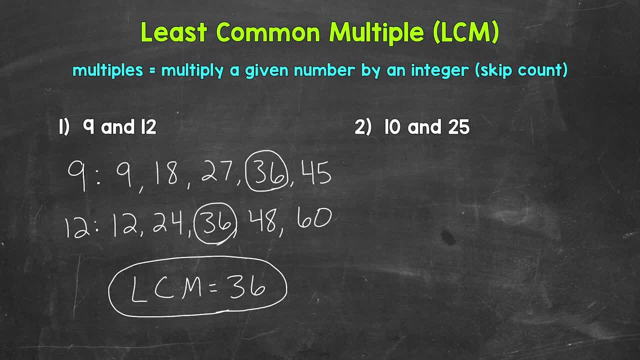 Although we only have one common multiple in our lists, as is 36, we can always extend multiples lists, So we can always keep going to find more common multiples. Remember: multiples are endless, So that means common multiples are Endless. 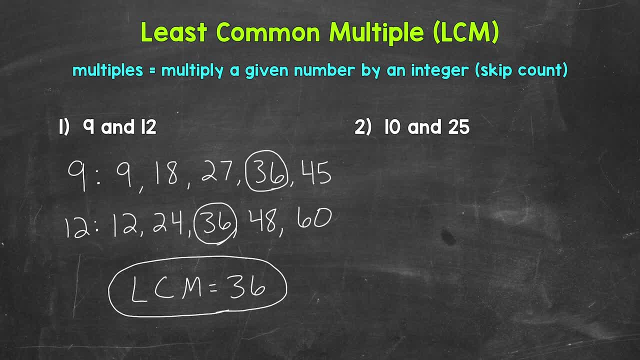 So that's just something to think about. when it comes to multiples, Let's move on to number 2, where we have 10 and 25.. Let's start with some multiples of 10.. So 10 times 1 is 10.. 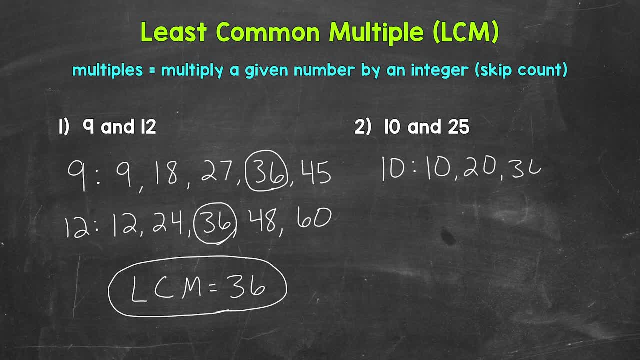 10 times 2 is 20.. 10 times 3 is 30.. 10 times 4 is 40., And then 10 times 5 is 50. So 10, 20,, 30., 40,, 50,, so on and so forth. 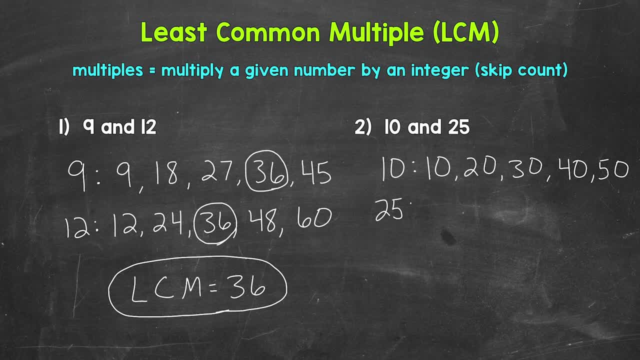 Now let's list the first five multiples of 25.. So 25 times 1 is 25.. 25 times 2 is 50.. 25 times 3 is 75.. 25 times 4 is 100.. And then 25 times 5 is 125.. 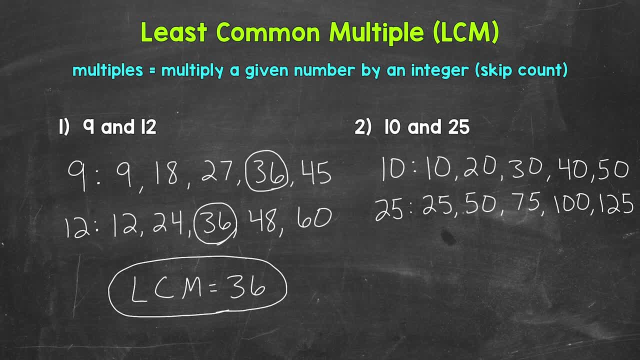 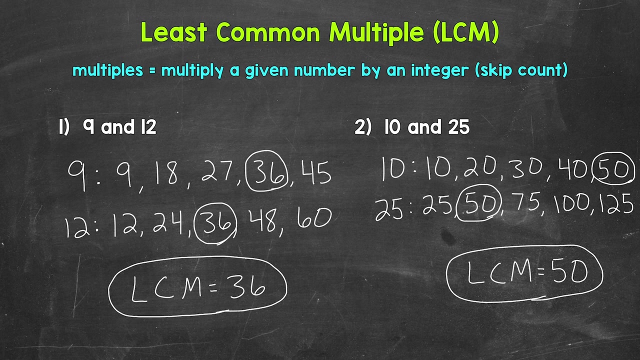 Now that we have some multiples listed, we can look for common multiples And specifically the least common multiple. Well, 50 is a common multiple And it happens to be the least common multiple, So the LCM is 50.. The least common multiple of 10 and 25 is 50.. 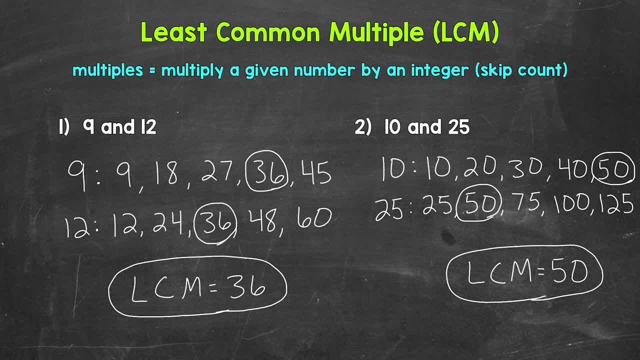 So there are two examples of finding the least common multiple by listing some multiples of the given numbers. Let's move on to finding the least common multiple of 10 and 25.. Here are some examples of finding the least common multiple by using prime factorization. 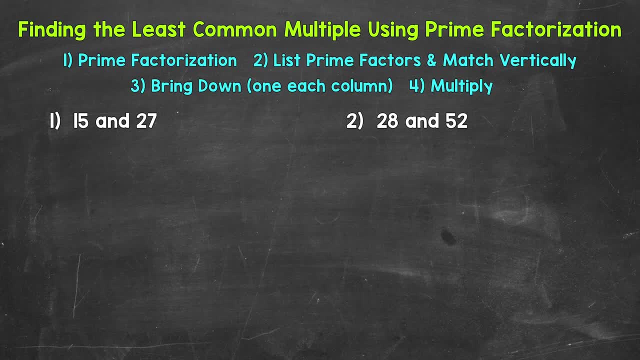 Here are our examples for finding the least common multiple by using prime factorization. Now, I like using this strategy and find it helpful when working with numbers that are a little larger in value and not as simple to work with. For example, the strategy of listing out multiples of numbers in order to find the LCM can be kind of boring. 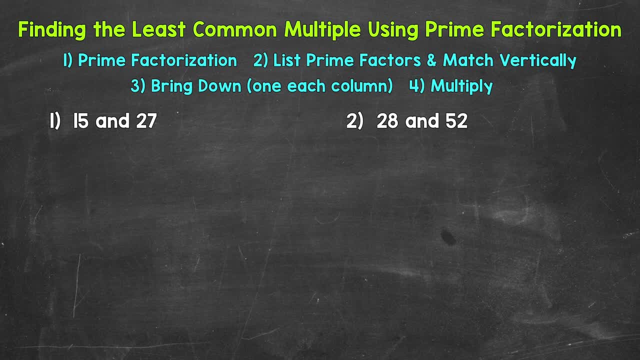 It can be kind of difficult and time-consuming when working with larger numbers in value. So this is a different approach, a different strategy to be familiar with when it comes to finding the least common multiple. Let's jump into our examples, starting with number 1, where we have 15 and 27.. 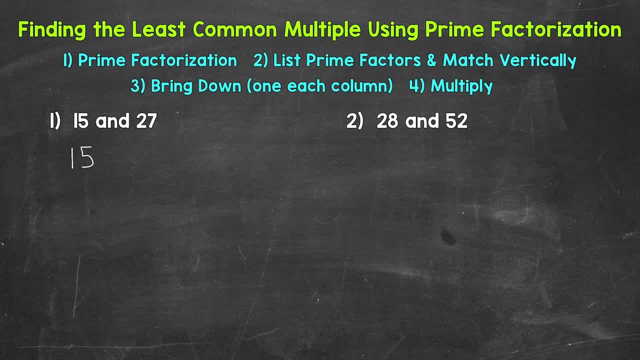 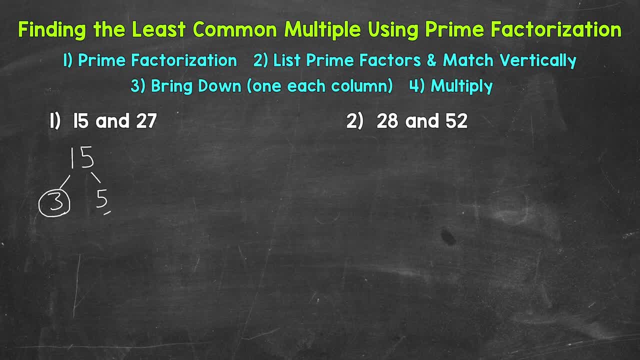 And 3,, 17, and 5.. And 3,, 17, and 5.. Now, 3 is prime, so we are done there, And 5 is prime, so we are done there as well, And that's the prime factorization of 15.. 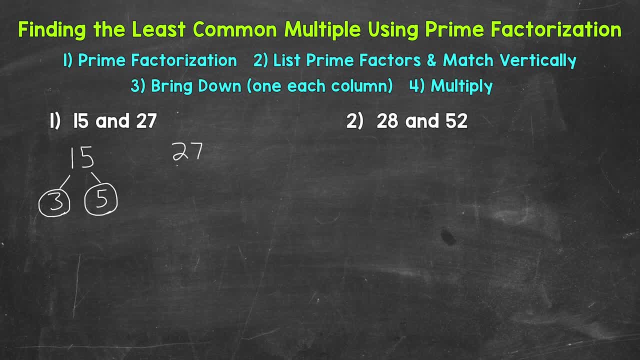 We can't break that down any further. Now we have the prime factorization of 27.. Now we have the prime factorization of 27.. Let's start with the factors of 3 and 9.. are factors of 27.. 3 is prime, so we are done there. but we can break 9 down. 3: 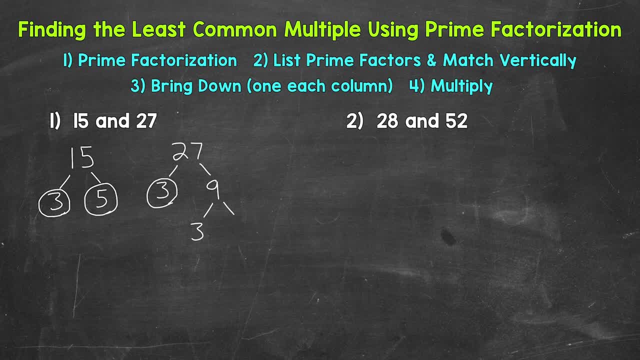 times 3 equals 9.. So 3 is a factor of 9.. 3 is prime. so we are done there and there, And that's the prime factorization of 27.. We can't break that down any further Now. 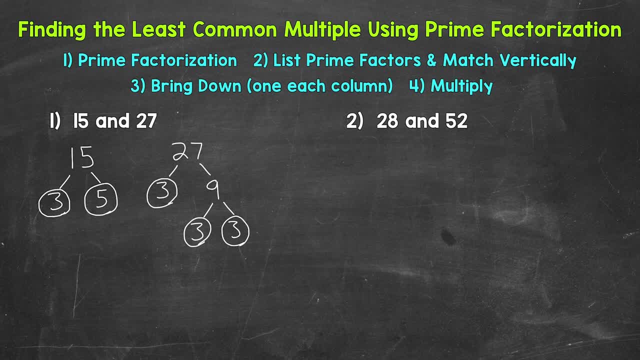 we're ready to move to the next step. So we need to list the prime factors of 15 and 27 and match them vertically. Let's see what this looks like Starting with 15.. So our prime factors from the prime factorization are 3 and 5, or 3 times 5.. Now for 27.. So 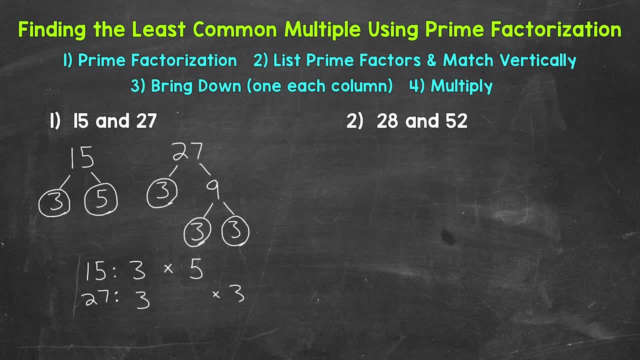 we have 3 times 5.. 3 times 3. And you'll notice that big gap underneath the 5. there We are matching numbers vertically. 27 does not have a prime factor of 5, so I left that blank underneath the. 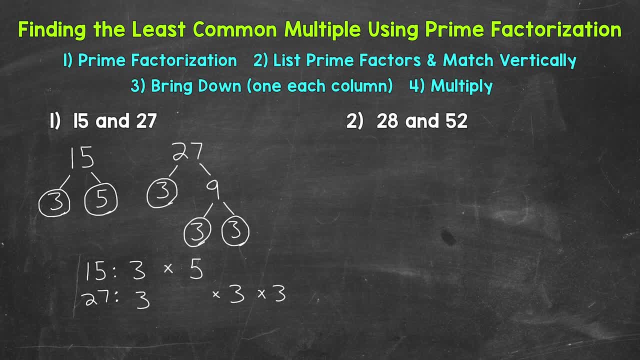 5. Now that we have our prime factors listed and matched vertically, we move on to the next step, where we bring down, And I like to draw a line underneath here in order to separate these steps. So this is a column And although we have two 3s here, this is a column of 3s. 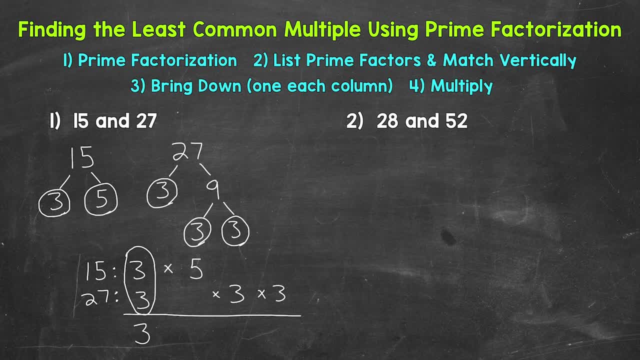 So we just bring 1 down. We have a 3 to represent that column of 2, 3s Times. We have a column of 5 here Times. We have a 3 here Times, Another 3 here. 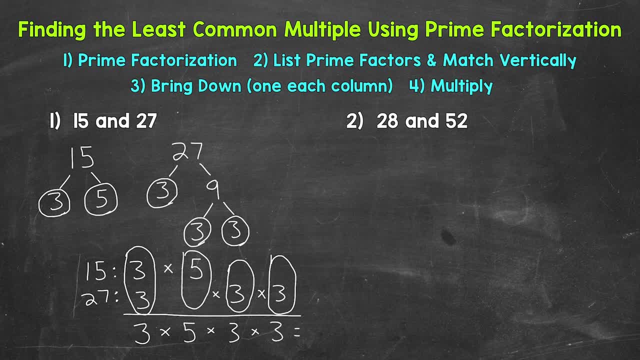 And so let's just add that UV 0.5 to V, 0.5 to V- Again adding more V V's a little bit online. We need a 4 and a 4. So 12 does not matter. We just need a 2 there. So this is a number, and 1 and a 10.. 3, 0.5 is. we don't have a prime factor. So now on to our prime factor: 5 times 5 and 5 is: 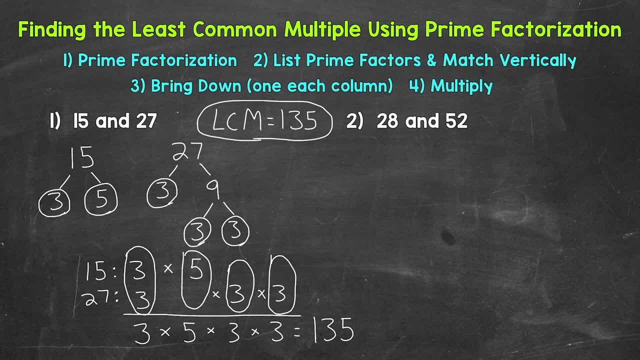 15 times 3.. Huh, Scratch here. Suppose we ended up with three times 5 times 3 times 3 and by multiplying these we get our least 135.. Let's move on to number two, where we have 28 and 52.. Let's start with the prime factorization. 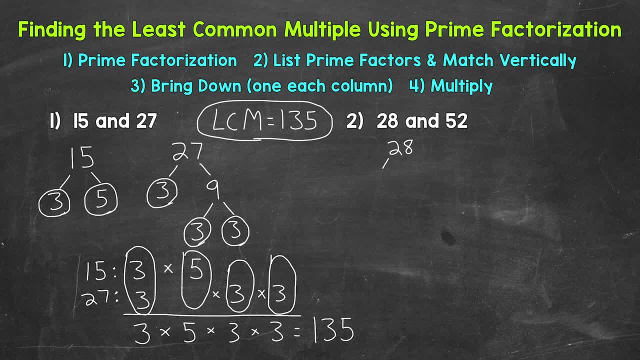 of 28.. Now, 2 times 14 equals 28, so let's start with those factors. 2 is prime, so we are done there. 14, we can break down 2 times 7, equals 14, so 2 and 7 are factors of 14.. 2 is prime, so we are. 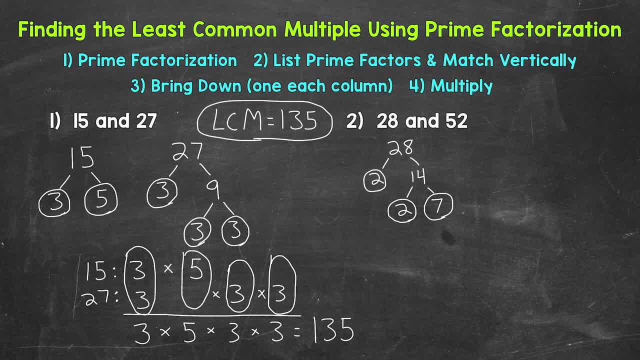 done there, and 7 is prime as well. so we are done there And that's the prime factorization of 28.. We can't break that down any further. Now we need the prime factorization of 52.. Let's start with the factors of 2.. 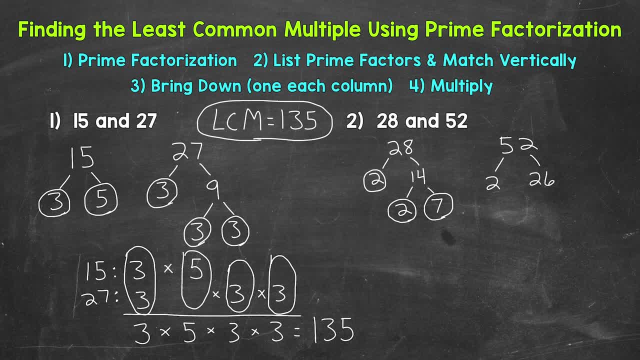 2 times 26 equals 52, so 2 and 26 are factors of 52.. 2 is prime, so we are done there. 26, we can break that down, 2 times 13, equals 26, so 2 and 13 are factors of 26.. 2 is prime, so we are done. 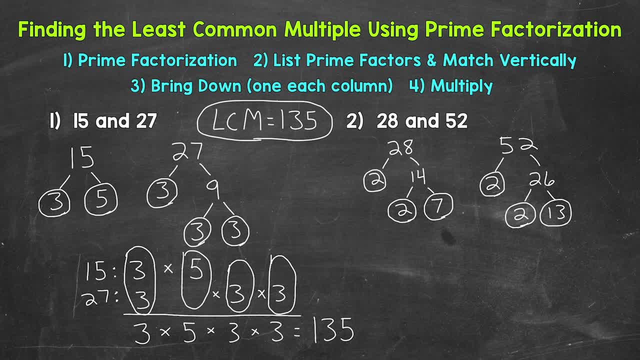 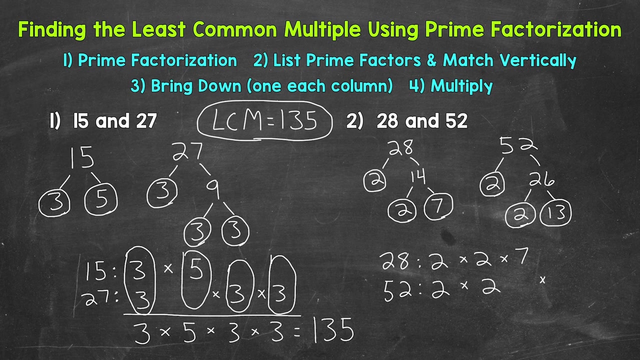 there and 13 is prime as well. so we are done there, And that's the prime factorization of 26.. prime factorization of 52.. We can't break that down any further Now. we need to list the prime factors and match them vertically. For 28, we have 2 times 2 times 7.. For 52, we have 2 times 2 times. 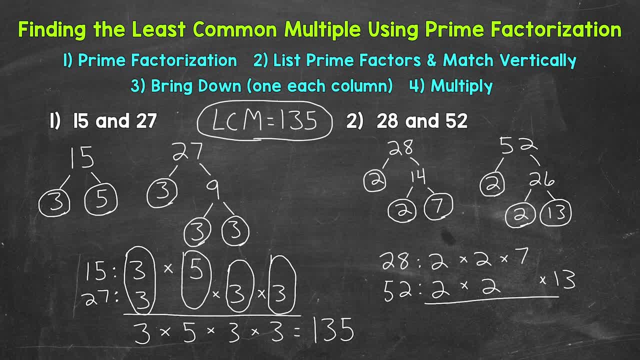 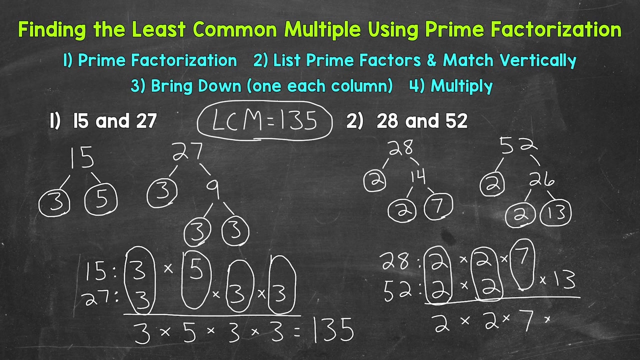 13.. Now we need to bring down. So we have a column of 2s here, So let's bring down a 2 to represent that column times. another column of 2s, So let's bring another 2 down. times 7 times 13.. 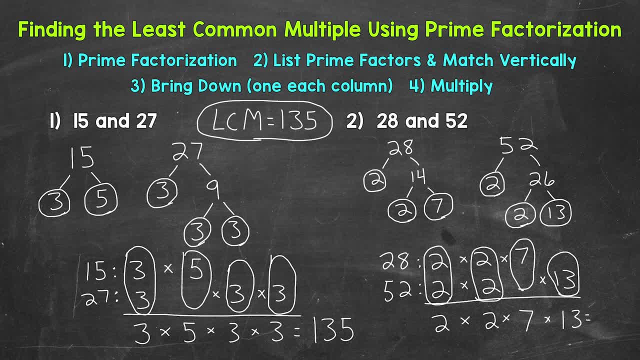 So we have 2 times 2 times 7 times 13 to get our least common multiple. We have 2 times 2, which is 4 times 7, is 28 times 13.. Well, I'm not sure what 28 times 13 is, So let's come to the side here. 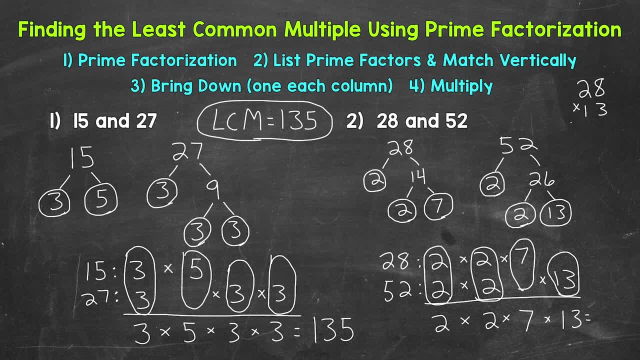 and multiply 28 times 13. We will start with 3 times 8, which is 24.. 3 times 2 is 6 plus 2 is 8.. We are done here and done here. We need a 0.. Now we have 1 times 8. 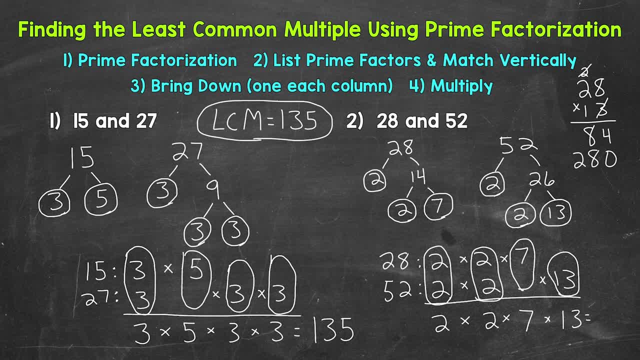 which is 8, and then 1 times 2 is 2.. Let's add: 4 plus 0 is 4.. 8 plus 8 is 16, and then 1 plus 2 is 3.. So we get 364.. 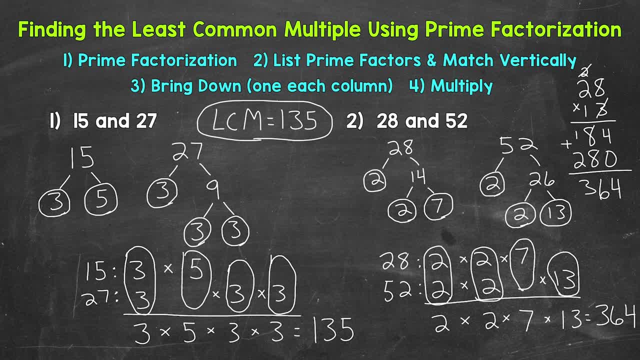 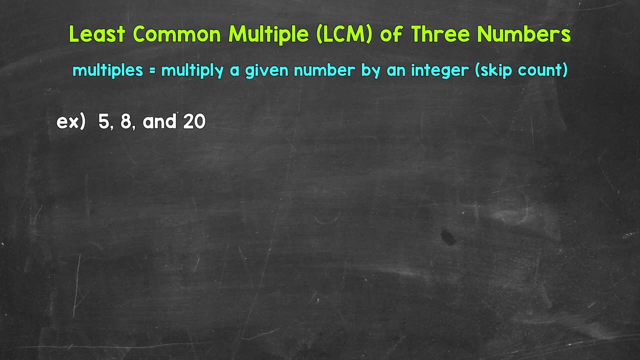 So the least common multiple of 28 and 52.. Let me squeeze this in here- is 364.. So there's how to find the least common multiple using prime factorization. Let's move on to finding the least common multiple of three numbers. Here is our example for finding the: 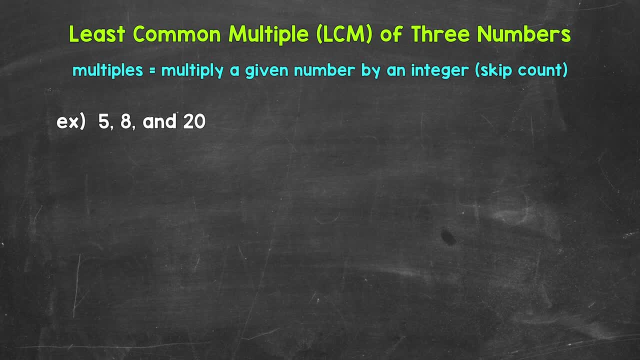 least common multiple of three numbers, And in this example we will use the strategy of listing out some multiples of the given numbers. Let's jump into our example, where we have 5,, 8, and 20.. So let's find the least common multiple. 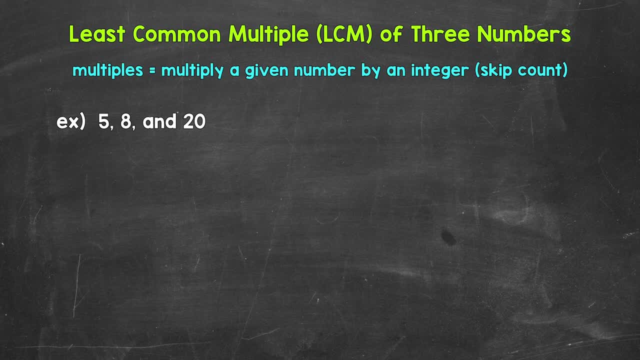 between these three numbers. Let's start with some multiples of 5.. So 5 times 1 is 5.. 5 times 2 is 10.. 5 times 3.. 5 times 4 is 20.. And 5 times 5 is 25.. So you can see that we just skip counted by 5 to list. 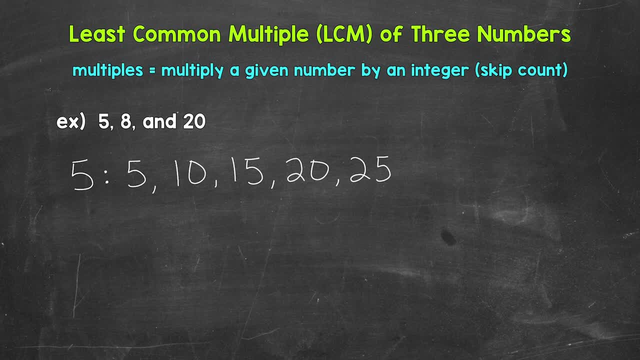 those multiples of 5.. 5,, 10,, 15,, 20,, 25, so on and so forth. Now I stopped at 25 because multiples go on forever, They are endless, They are infinite. My suggestion is to list 4 or 5 multiples of each number when looking for the least common. 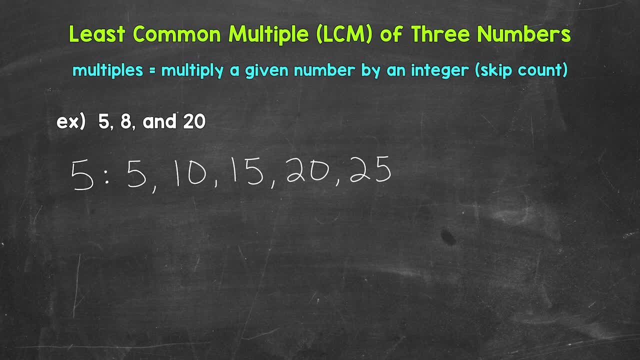 multiple. So list 4 or 5 for each number, Look for any in common, specifically the least common multiple, And if you don't have any in common, you can always extend the multiples lists. Now let's list the first 5 multiples of 8.. 8 times 1 is 8.. 8 times 2. 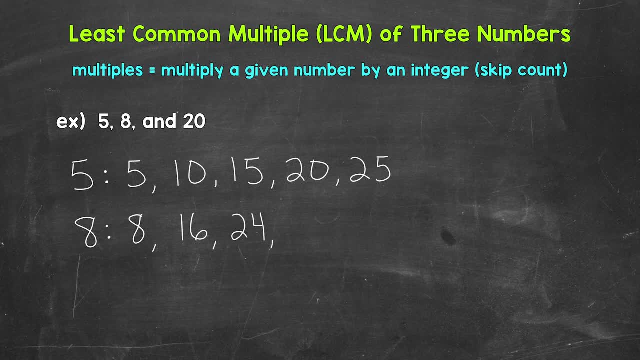 is 16.. 8 times 3 is 24.. 8 times 4 is 32.. And then 8 times 5 is 40. So so on and so forth. And then, lastly, let's list the first 5 multiples of 20.. So 20 times 1 is 20.. 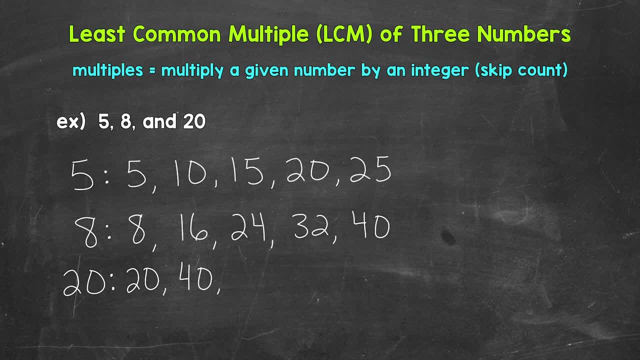 20 times 2 is 40.. 20 times 3 is 16.. 20 is 42.. 20 times 3 is 15 plus 1,겠습니다, 20 times 3 is 60.. 20 is 42.. And then 6 times 4 is 7, compared to a 4.. 8 x 4 equals 4, so they took the most common. 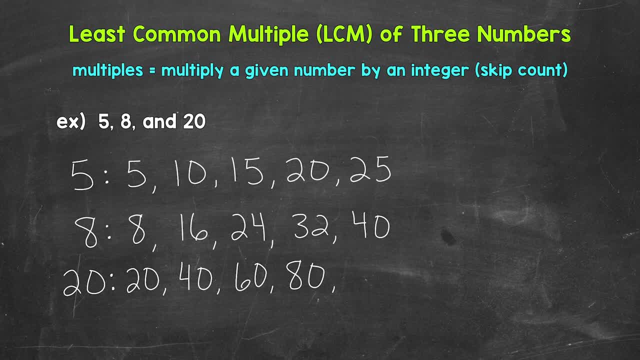 60, 20 times 4 is 80, and then 20 times 5 is 100.. So 20,, 40,, 60,, 80,, 100, so on and so forth. Now that we have some multiples listed for each number, we can look for common multiples. 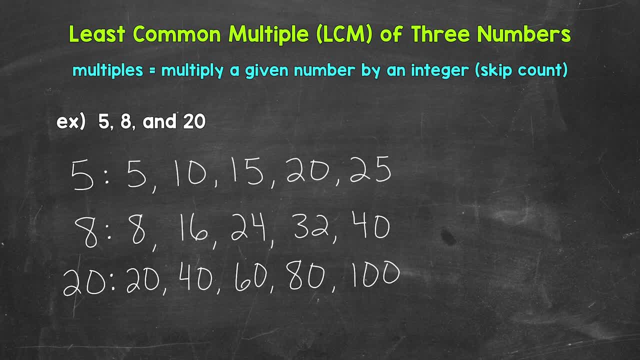 and specifically the least common multiple, so the smallest multiple in value that they all share. But, as of right now, we do not have any multiples that all three of these numbers share, so we need to continue our lists. Now as far as our lists of multiples, 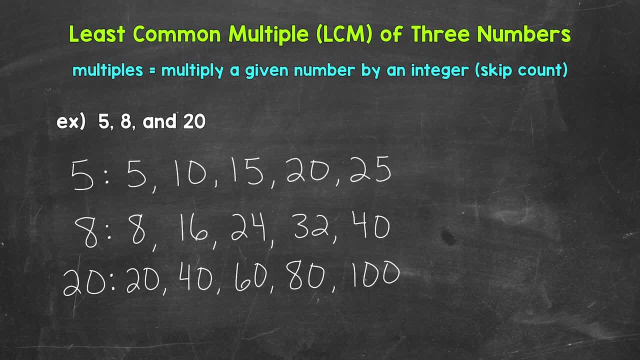 for the multiples of 20, we are at 100.. For the multiples of 8, we are at 40.. For the multiples of 5, we're only at 25.. So let's extend the list of multiples of 5.. So after 25,, 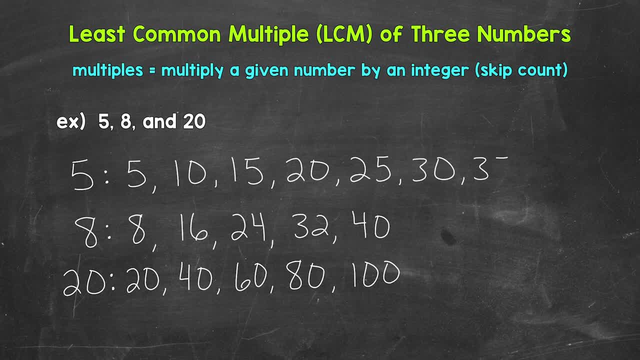 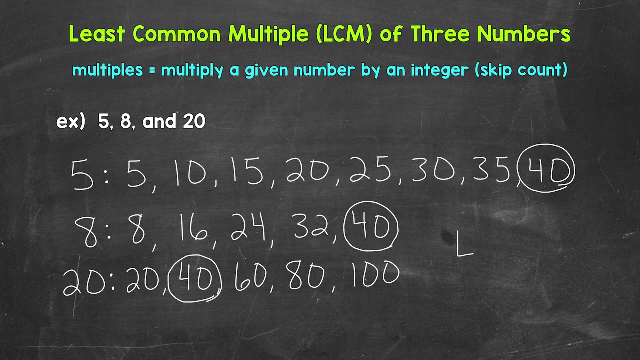 we have 30,, then 35, and then 40. Now 40 is going to be a common multiple, a multiple that all of our numbers share And, specifically, it's going to be the least common multiple. So, again, 40 is going to be our least common multiple. So the LCM, which stands for least. 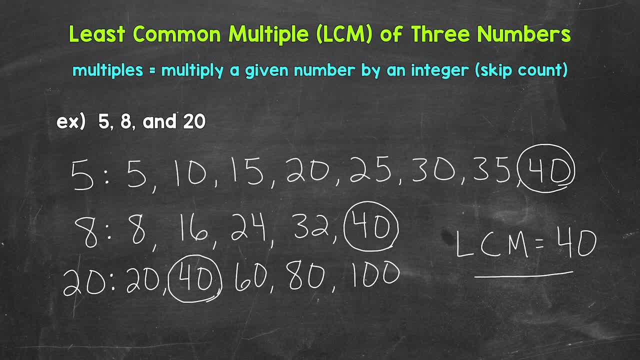 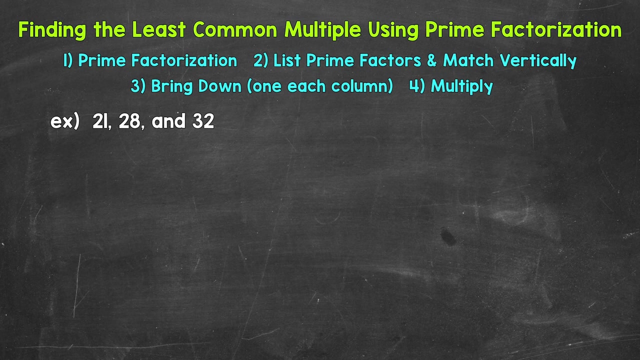 common multiple is 40.. So there's how we find the least common multiple of three numbers: by listing out some multiples of the given numbers. Let's move on to another example where we will use prime factorization. Here is our example for how to find the least common multiple of three numbers. 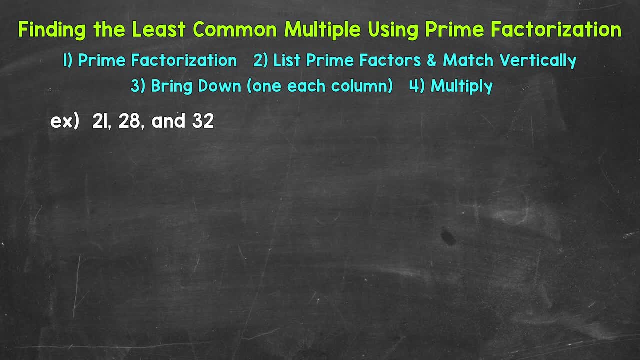 using prime factorization. Let's jump into our example where we have 21,, 28, and 32.. So we need to find the least common multiple of those three numbers. Let's start with the prime factorization of all three of our numbers, starting with 21.. 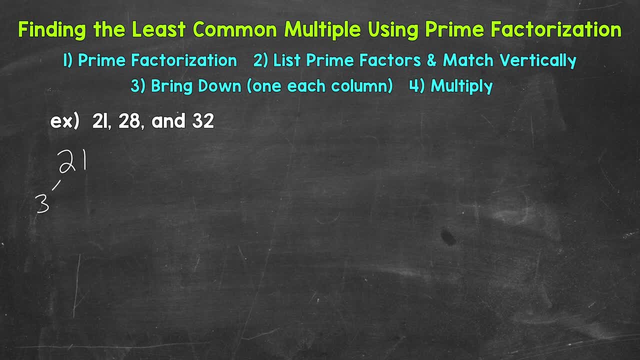 3 times 7 equals 21.. So 3 and 7 are factors of 21.. Now, 3 is prime, so we are done there. 7 is prime as well, So we are done there, And that's the prime factorization of 21.. We can't break that down. 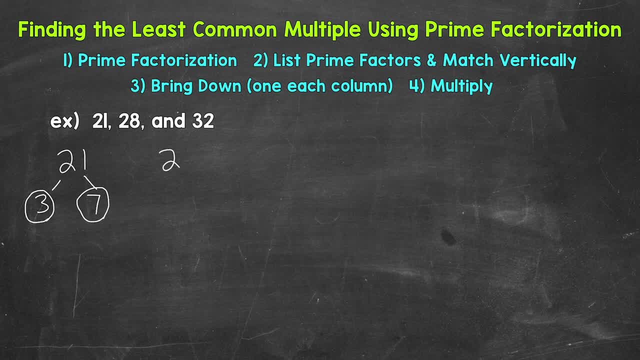 any further. Let's move on to 28.. 2 times 14 equals 28.. So 2 and 14 are factors of 28.. 2 is prime. so we are done there. 14, we can break down 2 times 7, equals 14.. 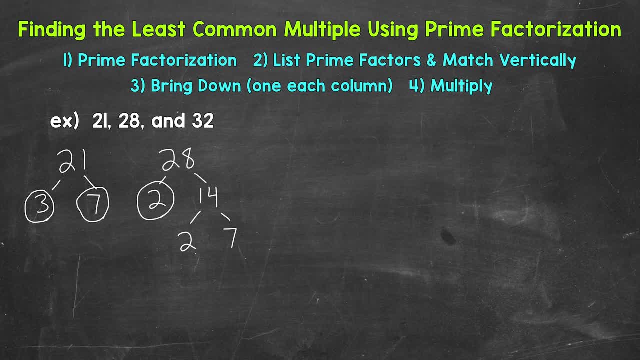 So 2 and 7 are factors of 14.. 2 is prime, so we are done there. 7 is prime as well, So we are done there, And that's the prime factorization of 28.. We can't break that down any further. Lastly, we have the prime factorization of 32.. 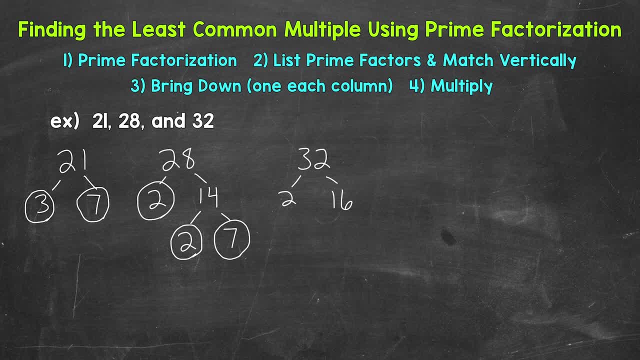 2 times 16 equals 32.. So 2 and 16 are factors of 32.. 2 is prime, so we are done there. 16, we can break down 2 times 8, equals 16. so 2 and 8 are factors. 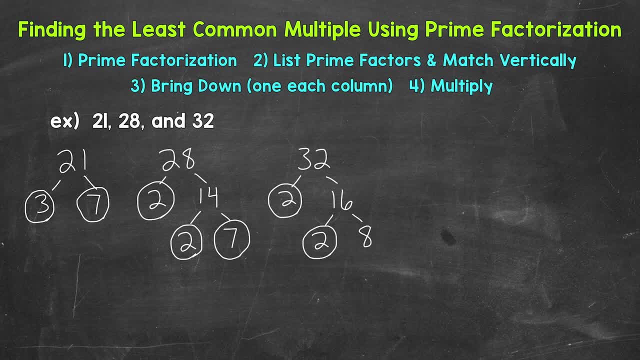 of 16.. 2 is prime, so we are done there. We can break 8 down further 2 times 4 equals 8, so 2 and 4 are factors of 8.. 2 is prime, so we are done there. We can break 4 down further 2 times 2. 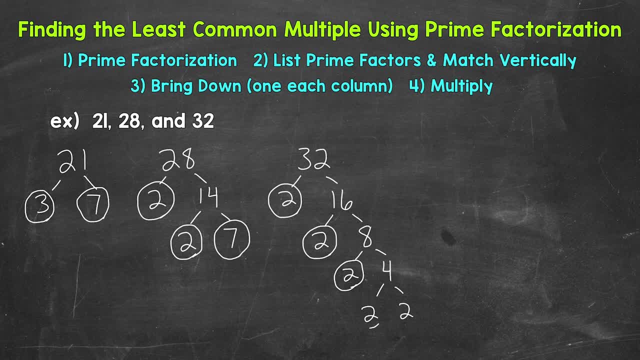 equals 4, so 2 is a factor of 4.. 2 is prime. so we are done there and there, And that's the prime factorization of 32.. We can't break that down any further, Now that we have the prime factorization. 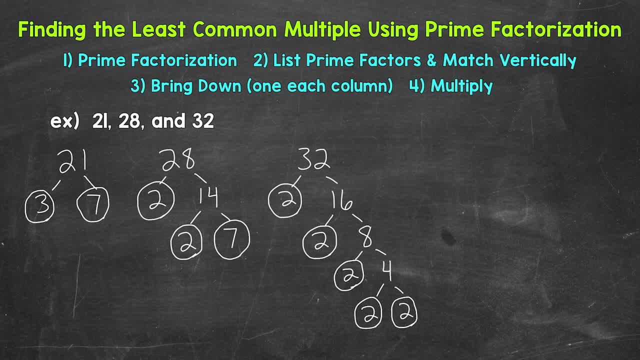 of all three of our numbers, we need to list the prime factors and match them vertically. Let's start with the prime factors of 21.. So 3 and 7.. 3 times 7 equals 21.. Now for the prime factors of. 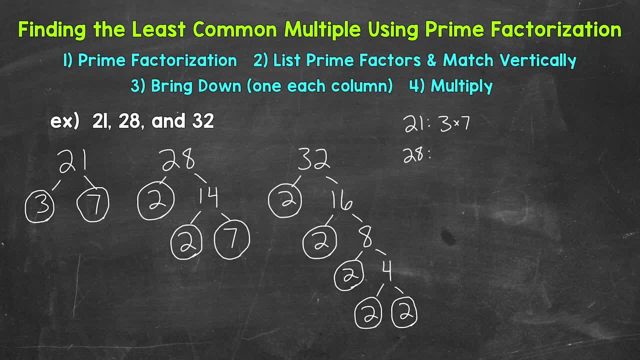 28. And I'm going to start with the prime factor of 7.. Since 21 also has a prime factor of 7, I'm matching the sevens vertically. Then we have the prime factors of 7.. Since 21 also has a prime factor of 7, I'm matching the sevens vertically. Then we have 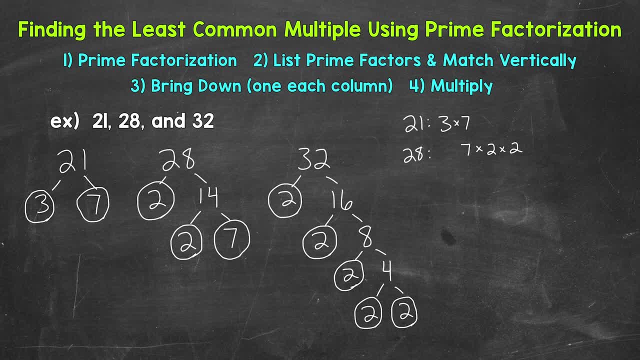 2 and 2.. So 7 times 2 times 2 equals 28.. And then, lastly, we have the prime factors of 32.. We have a 2 that we can match vertically, another 2 that we can match vertically, and then three more 2s, Now that we have our prime factors. 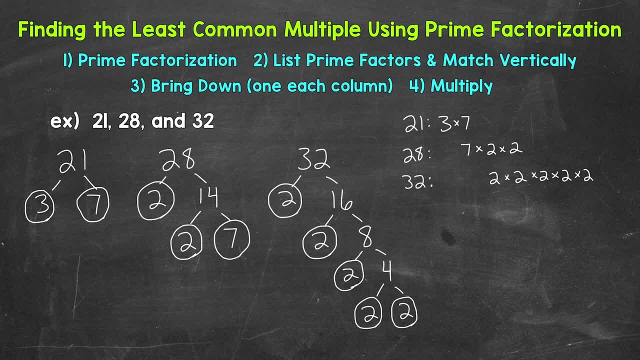 listed and matched vertically. we need to bring down a number to represent each column, And it's going to be 1 for each column. You'll see what this means as we go through this step. So I like to draw a line to separate our steps. 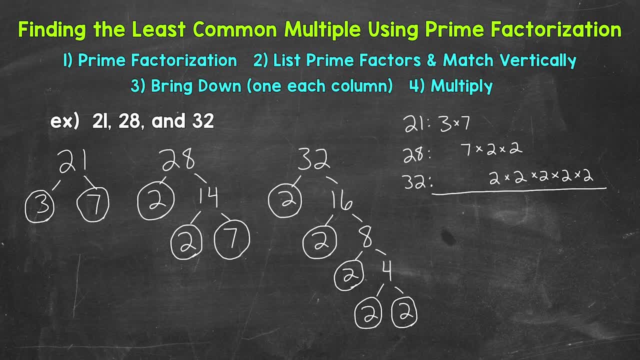 here And now again, we need to go through each column and bring down a number to represent that column. For example, we have a 3 column right here, Even though there's one 3, that's okay, We have a 3 column there, So let's bring down a 3 to represent it. 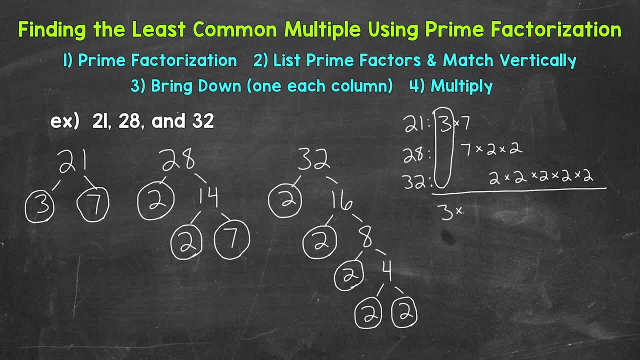 Let's bring down a 3 to represent that column Times. We have a 7 column here Now. there are two 7s there, but we only bring down one 7 to represent that column Times. Next we have a column of 2s, So bring down a 2 to represent that column And then another column. 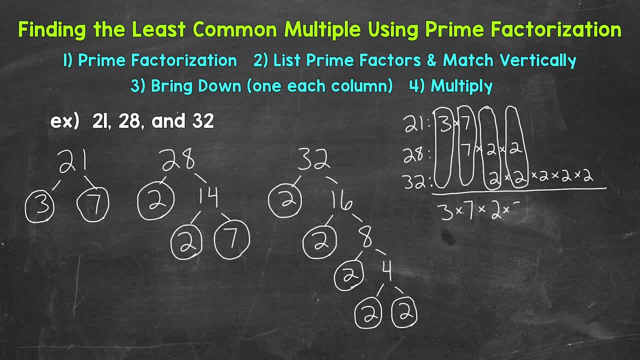 of 2s, So bring down another 2 to represent that column, And then another column of 2s, So bring down a 2 to represent that column Times. We have one 2 here, but it is a column. 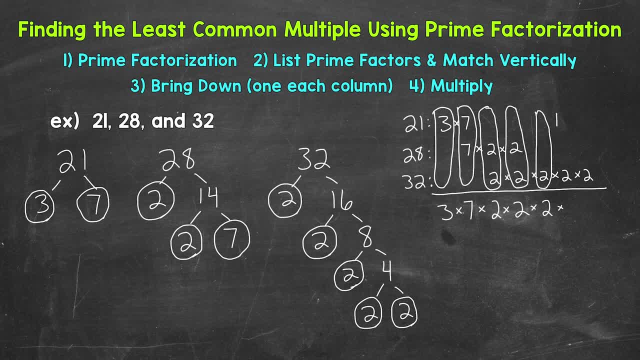 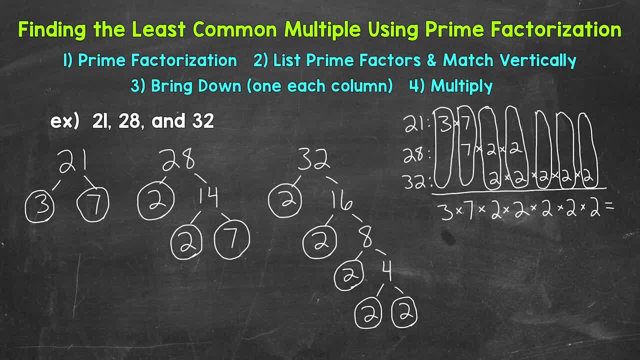 least common multiple. Now there are different ways to go about multiplying these numbers. For example, you can start with 3 times 7 and work your way from left to right. I'm going to start with this group of 5 2s right here. So we have 2 times 2 times 2 times 2. 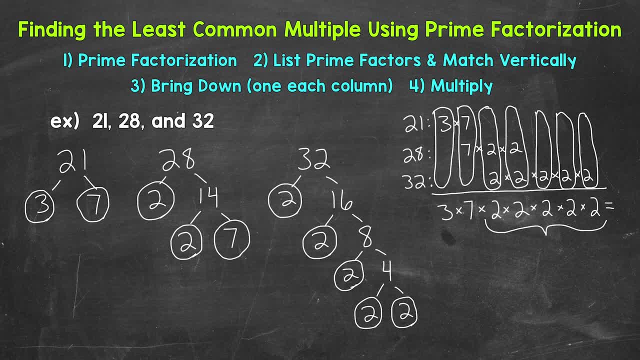 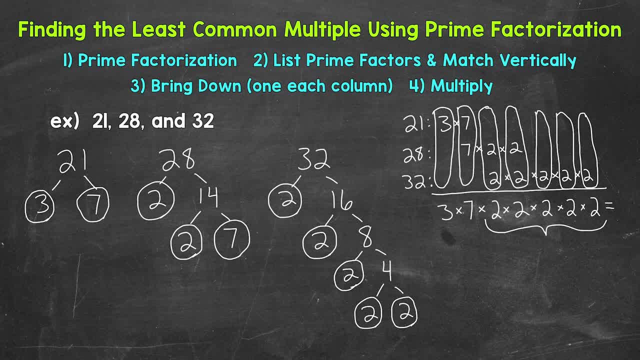 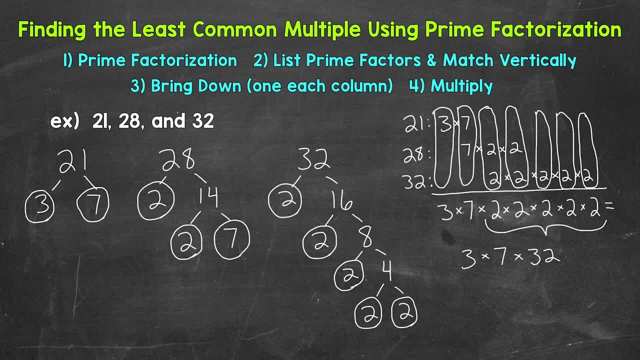 are different ways to go about multiplying these numbers. I'm just going to work from left to right, So I'll do 3 times 7 next, which is 21.. And then we have 21 times 32 for our last step. 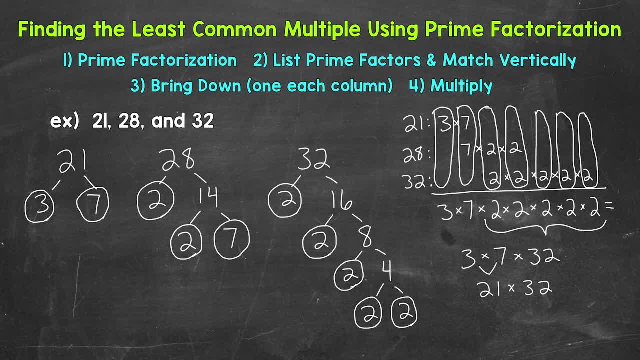 Now I'm not sure what 21 times 32 is, so I need to work this out off to the side. So 32 times 21.. I put the larger number in value on top. Let's multiply: 1 times 2 is 2.. 1 times. 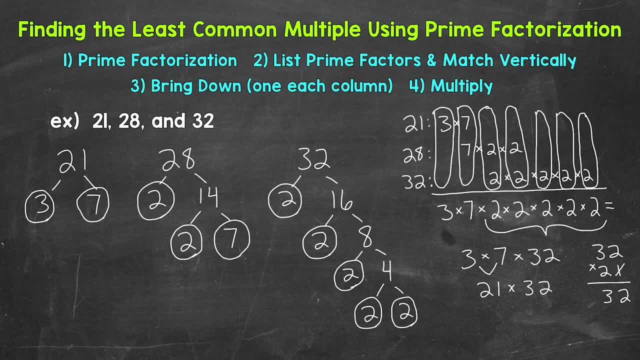 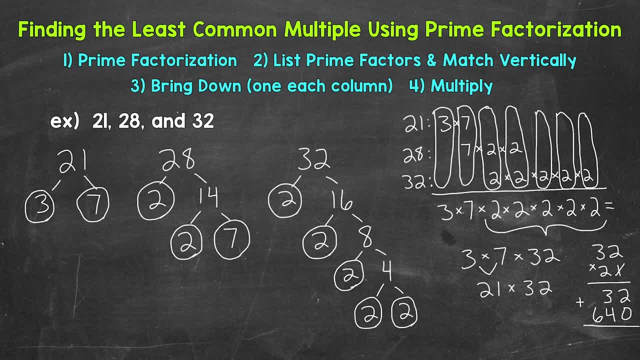 3 is 6.. Now we add 32 plus 640.. 2 plus 0 is 2.. 3 plus 4 is 7.. And then we have that 6.. So 672.. And that's our least common multiple. So I'll put an arrow there. So 3 times, 7 times.